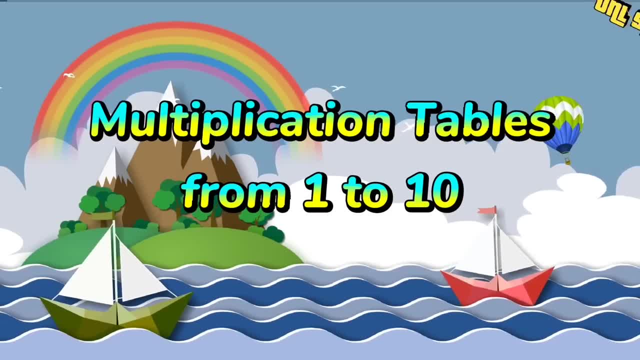 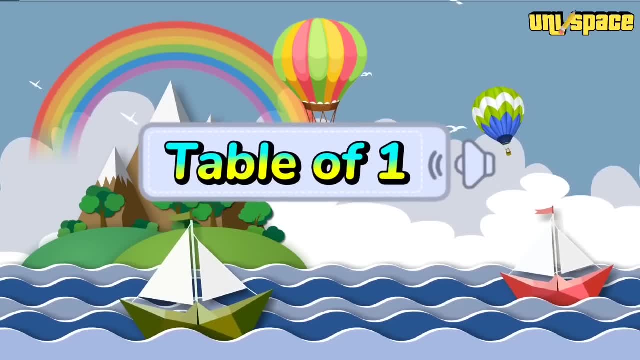 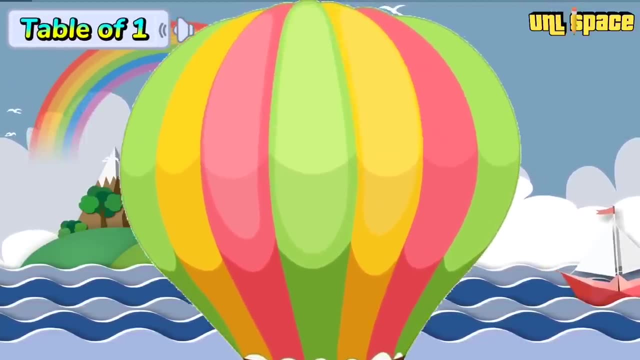 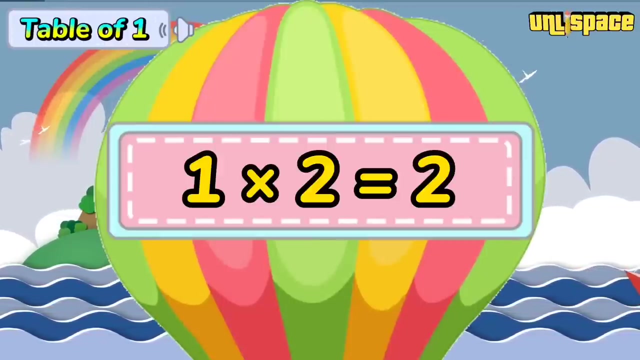 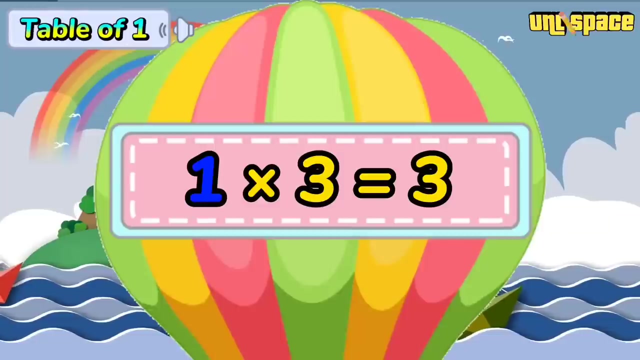 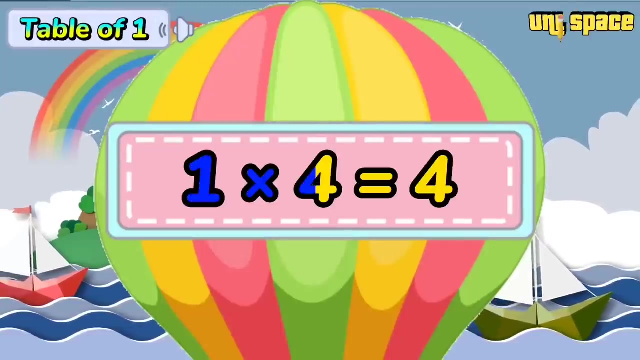 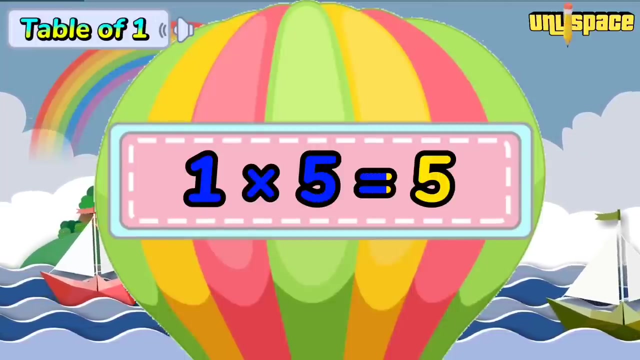 Multiplication Tables from 1 to 10. Table of 1. 1 x 1 equals 1. 1 x 2 equals 2. 1 x 3 equals 3. 1 x 4 equals 4. 1 x 5 equals 5. 1 x 6 equals 6. 1 x 7 equals 7. 1 x 8 equals 8. 1 x 9 equals 9. 1 x 10 equals 10. Table of 2. Table of 2. Table of 2. 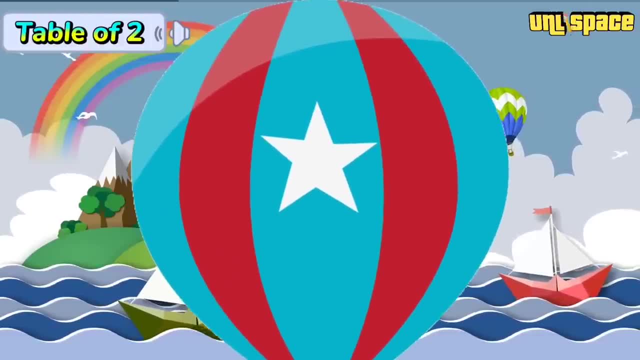 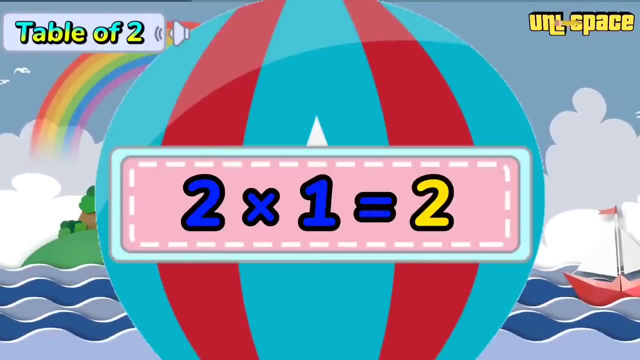 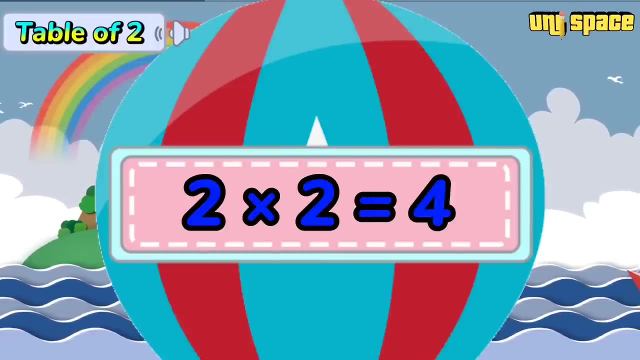 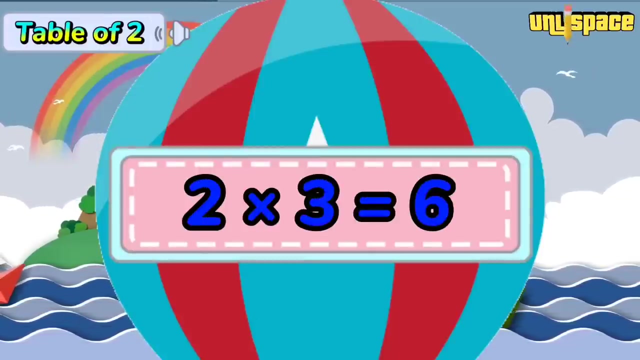 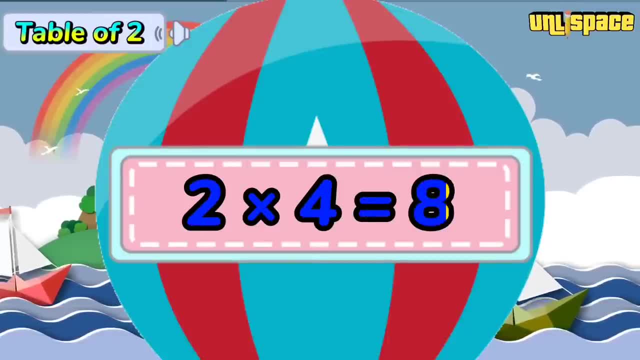 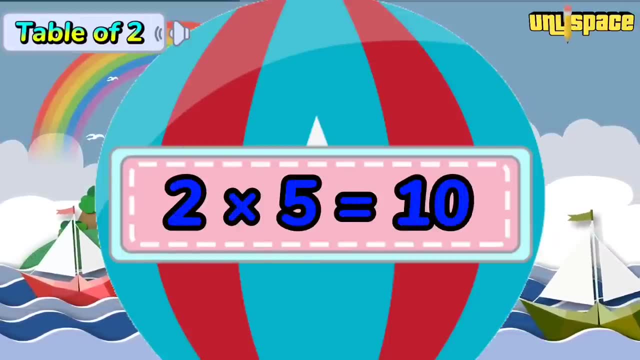 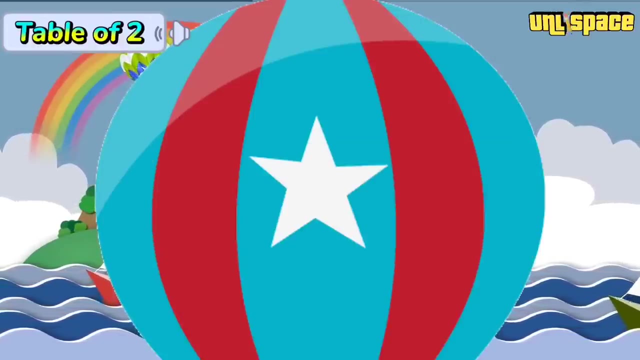 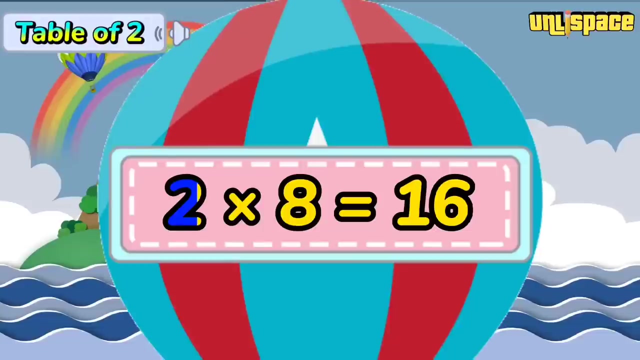 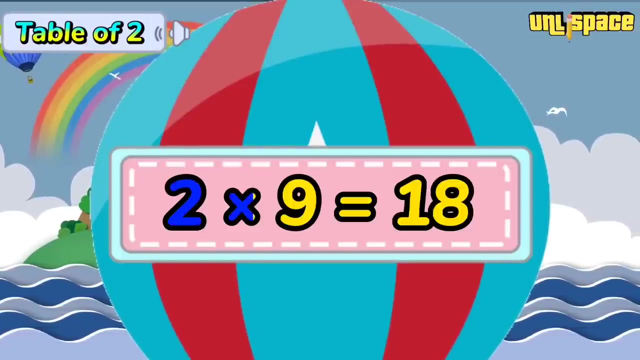 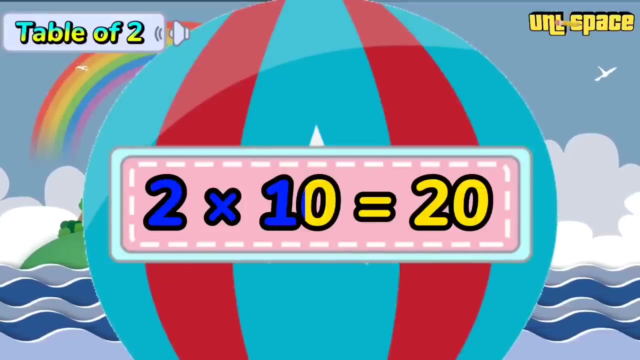 2 x 4 equals 8. 2 x 5 equals 10. 2 x 6 equals 12. 2 x 7 equals 14. 2 x 8 equals 16. 2 x 9 equals 18. 2 x 10 equals 20. 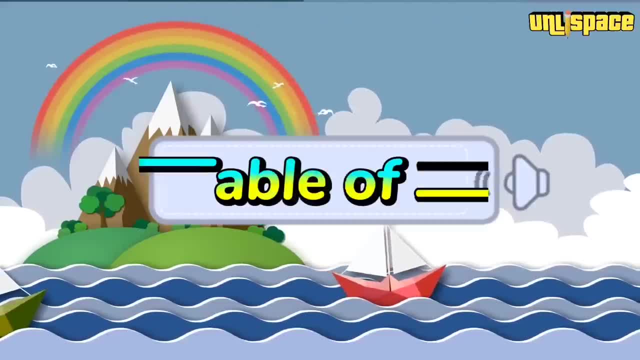 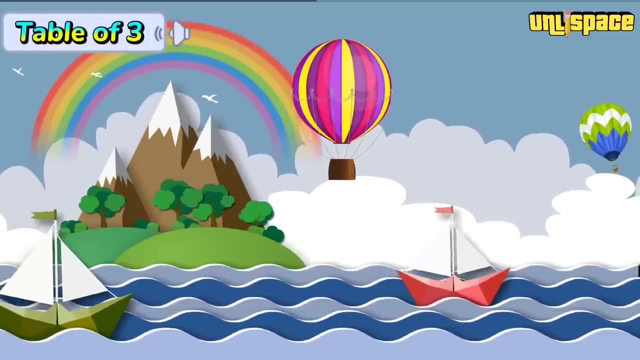 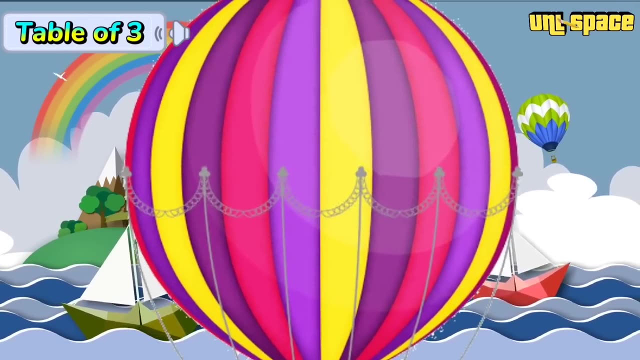 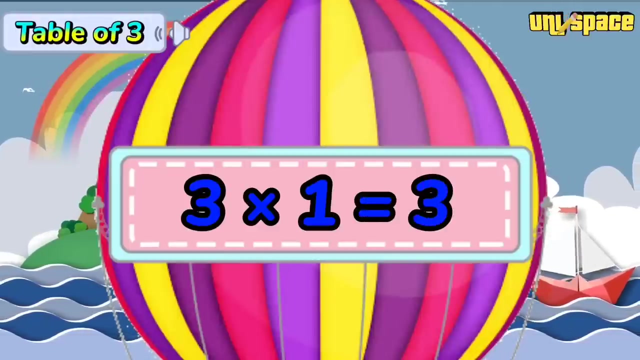 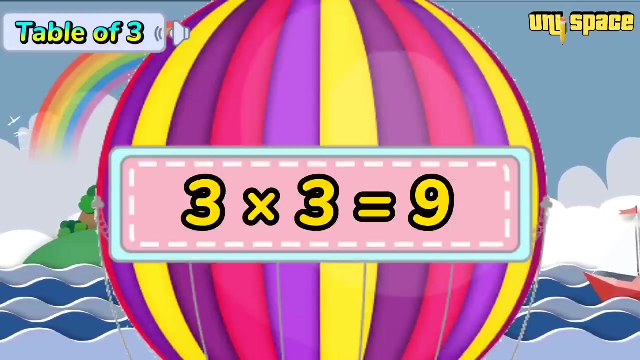 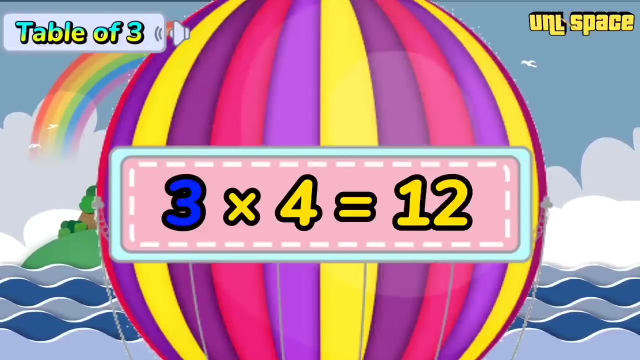 Table of Three. Table of Three: 3 x 1 equals 3. 3 x 2 equals 6. 3 x 3 equals 9. 3 x 4 equals 7. 3 x 4 equals 8. 3 x 4 equals 9. 3 x 4 equals 9. 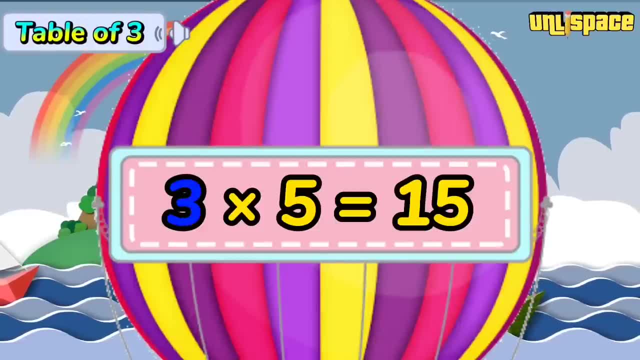 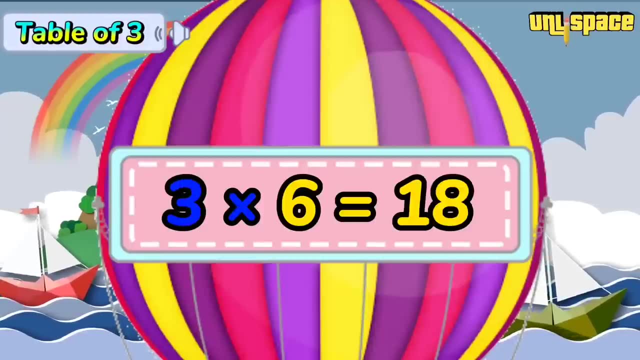 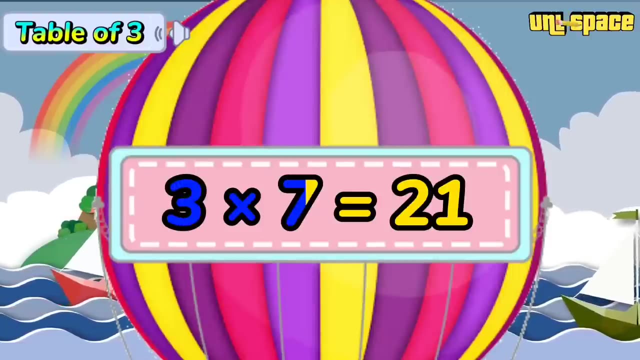 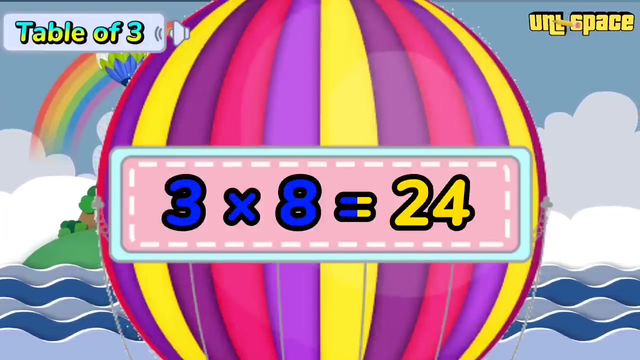 3 x 4 equals 12. 3 x 5 equals 15. 3 x 6 equals 18. 3 x 7 equals 21. 3 x 8 equals 24. 3 x 9 equals 20. 4 x 8 equals 21. 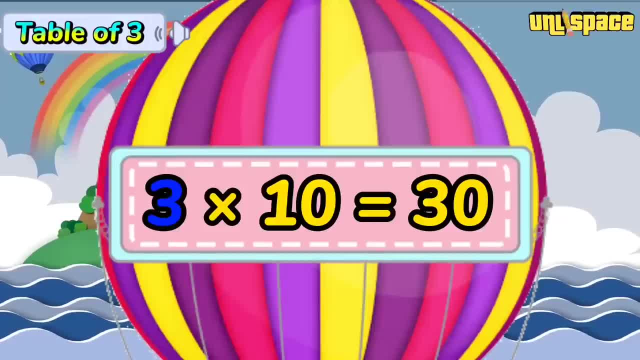 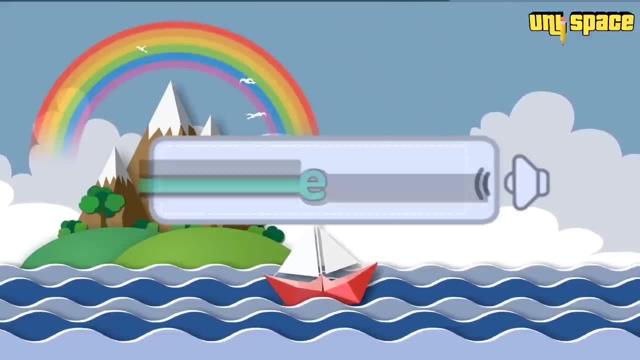 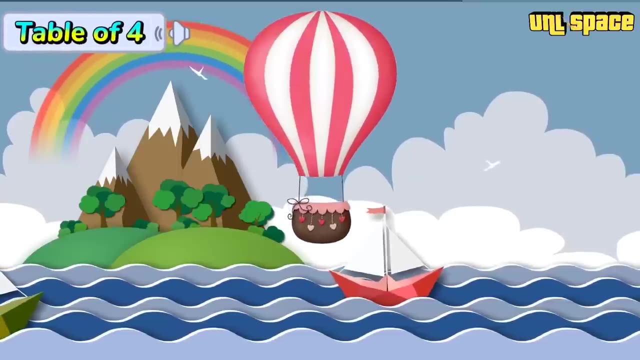 4 x 9 equals 19. 1 x 8 equals 9. 1 x 9 equals 24. 1 x 9 equals 24. 3 x 9 equals 27. 3 x 10. equalscendo Table of Four. 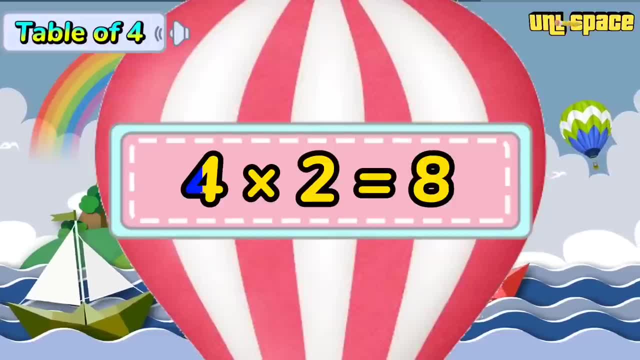 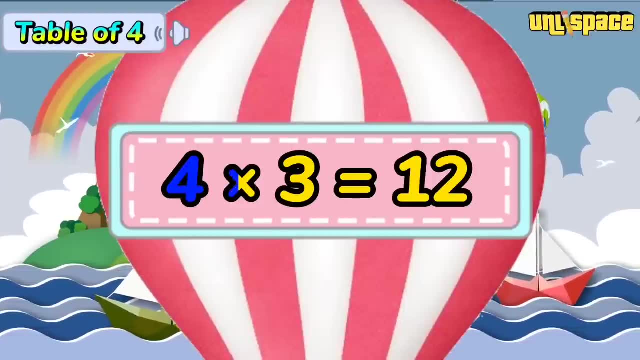 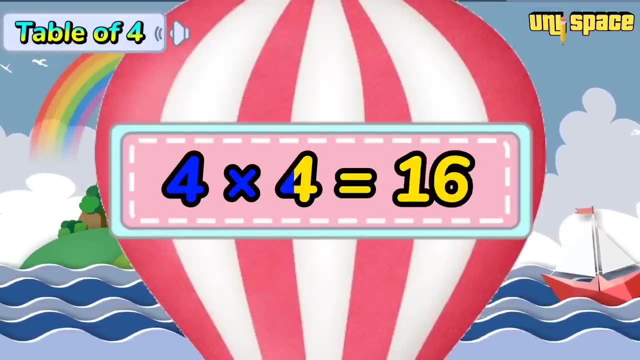 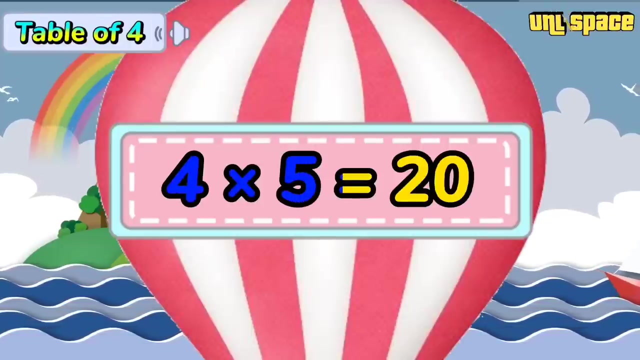 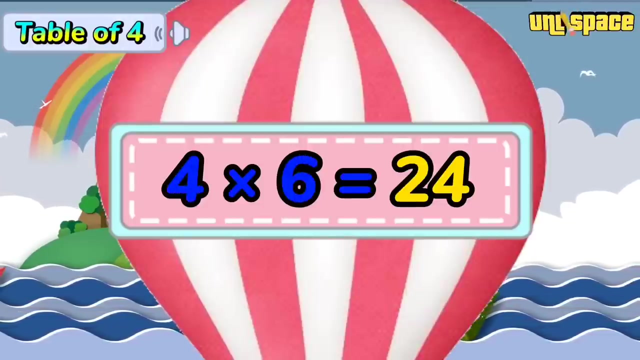 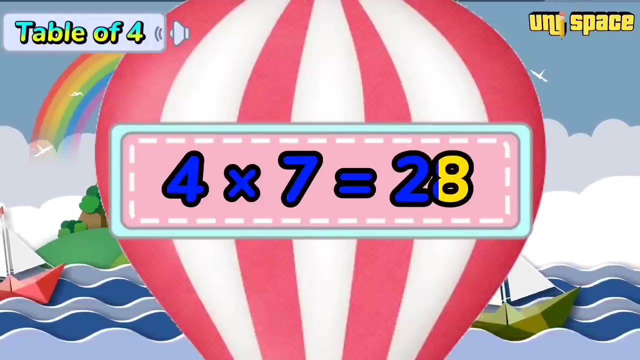 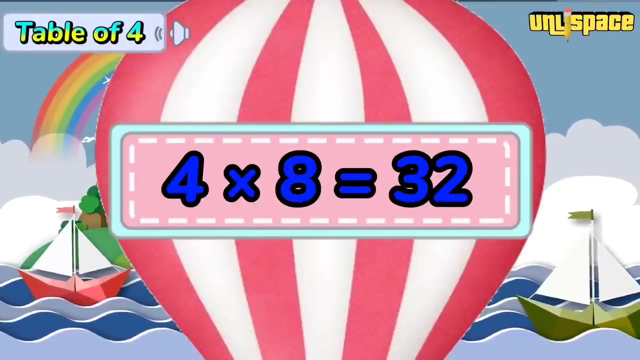 Table of Four. Table of Four. 4 x 1 equals 4, two equals eight. Four times three equals twelve. Four times four equals sixteen. Four times five equals twenty. Four times six equals twenty-four. Four times seven equals twenty-eight. Four times eight equals thirty-two. Four times nine equals thirty-six. 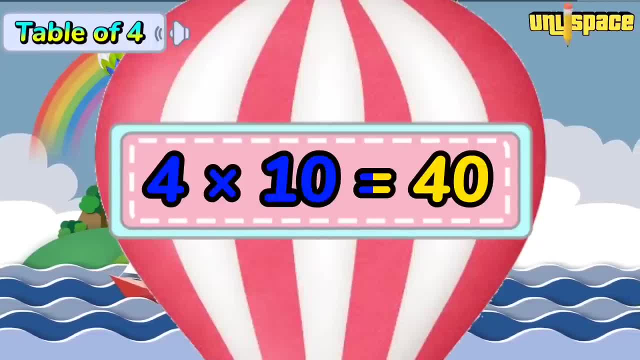 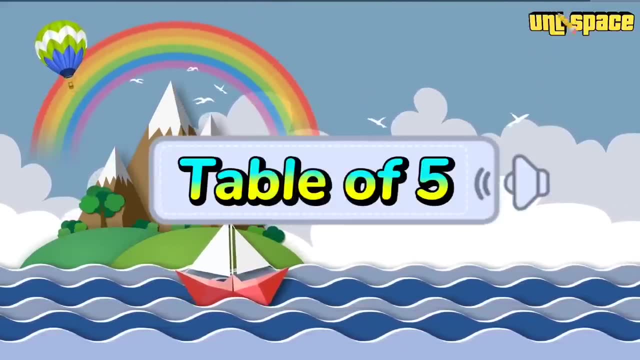 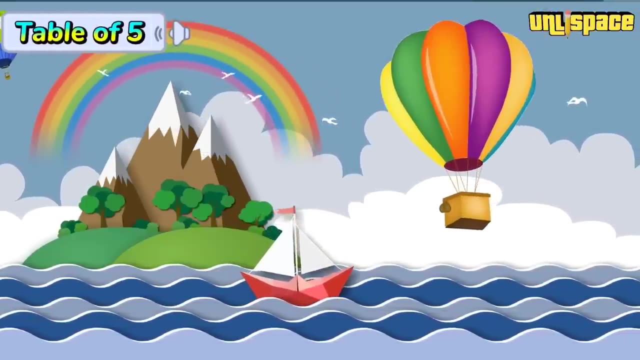 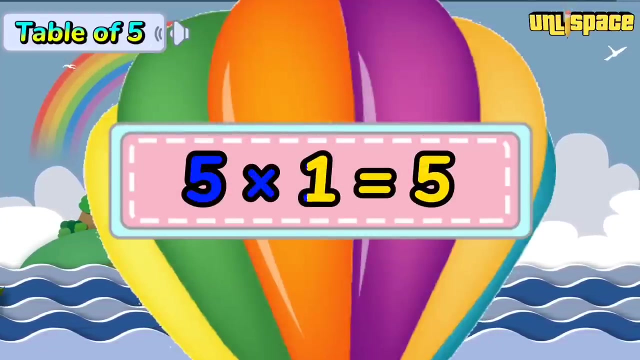 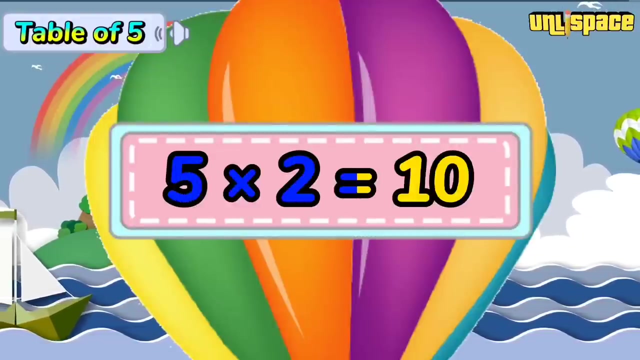 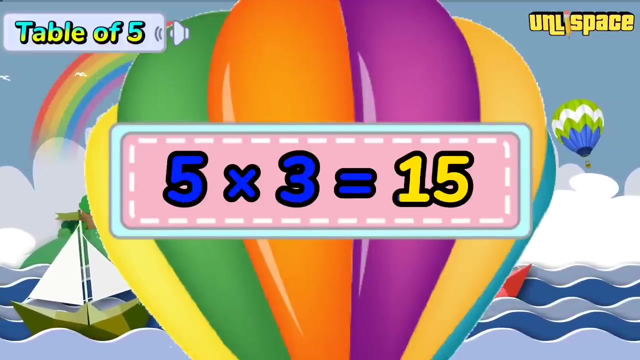 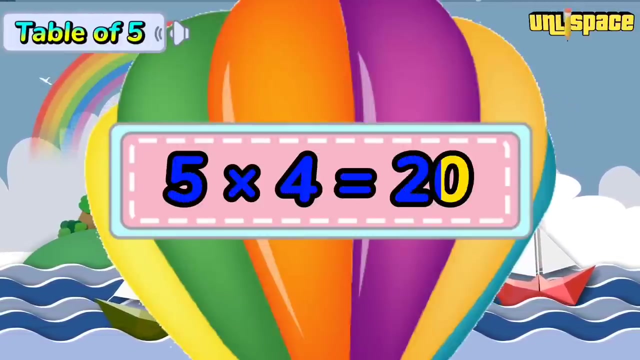 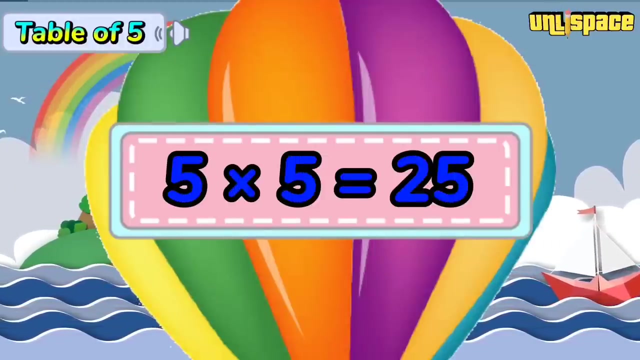 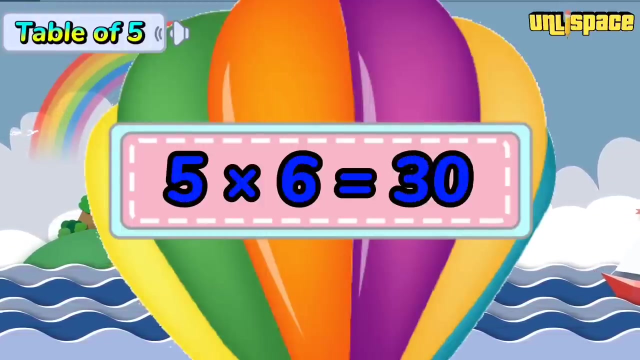 Four times ten equals forty. Table of five: Five times one equals five. Five times ten times two equals ten. Five times three equals fifteen. Five times four equals twenty. Five times five equals twenty-five. Five times six equals thirty. Five times six equals thirty. 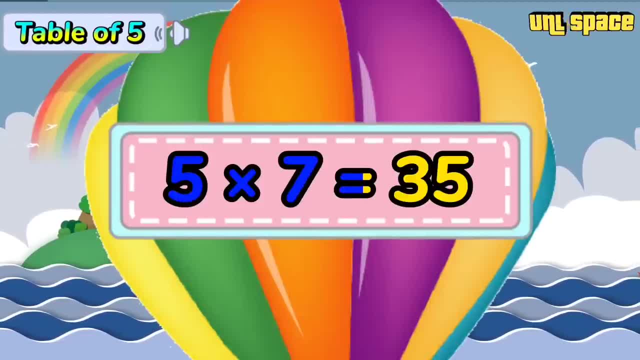 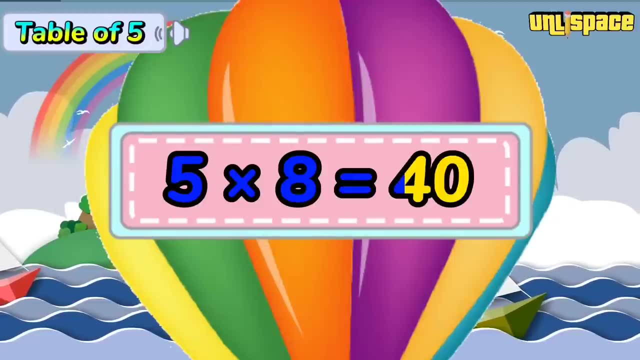 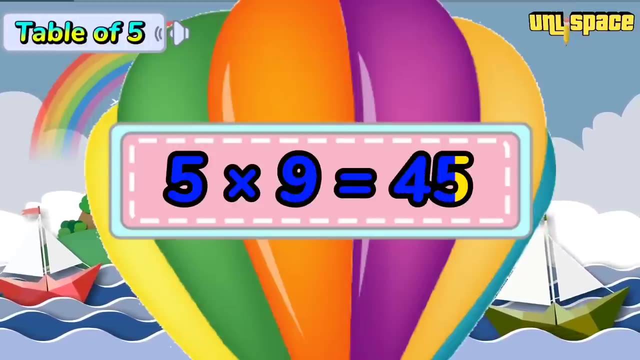 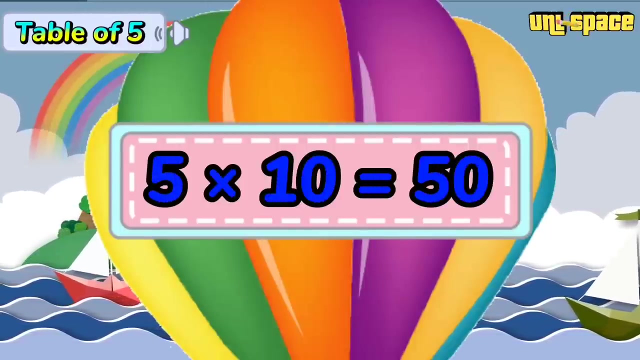 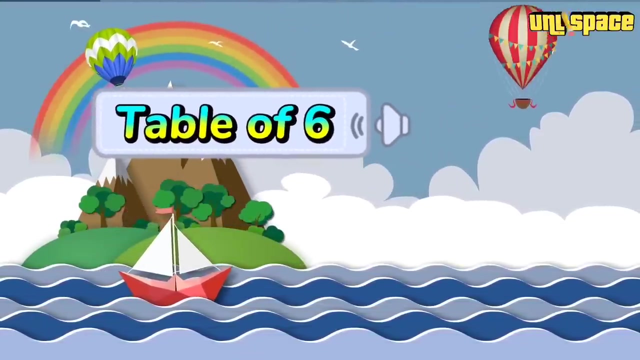 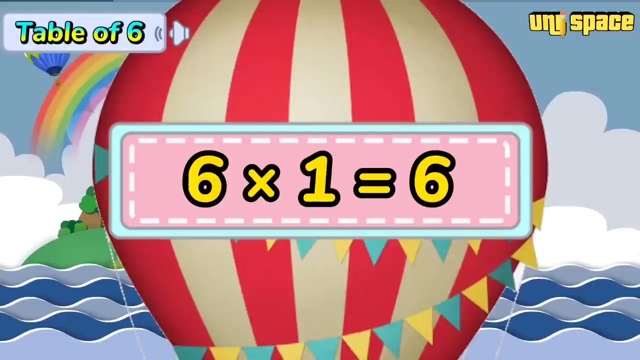 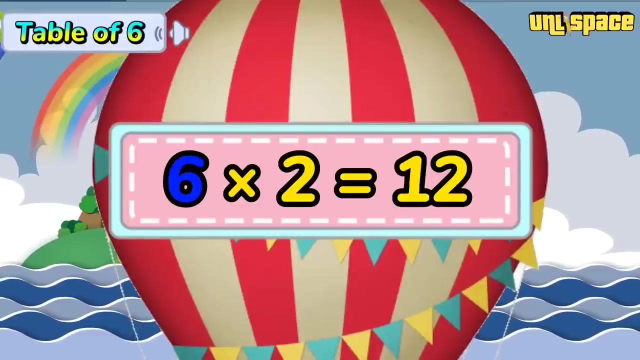 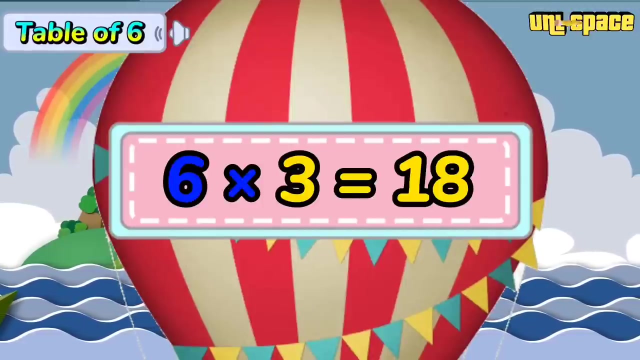 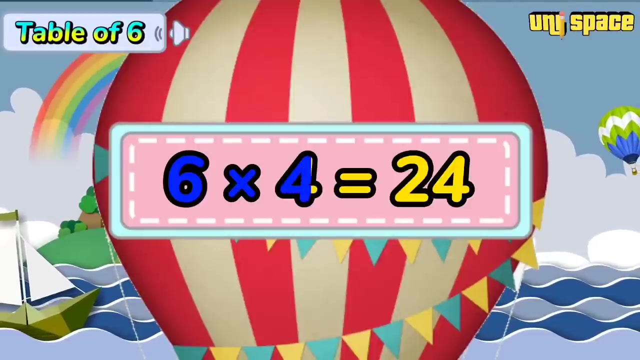 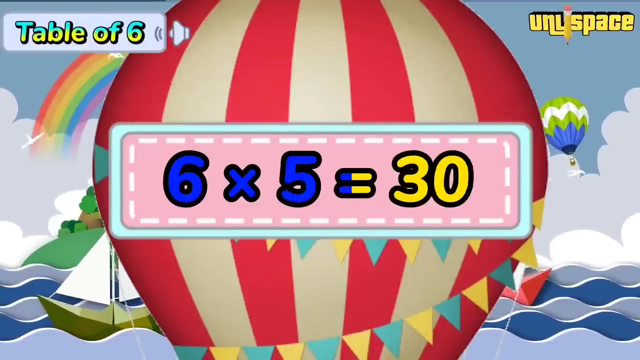 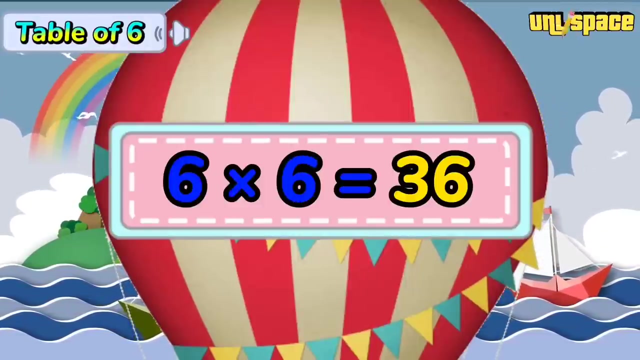 Five times seven equals thirty-five. Five times eight equals forty. Five times nine equals forty-five. Five times ten equals fifty. Table of six Six times one equals six. Six times two equals twelve. Six times three equals eighteen. Six times four equals twenty-four. Six times five equals thirty. Six times six equals thirty-six. 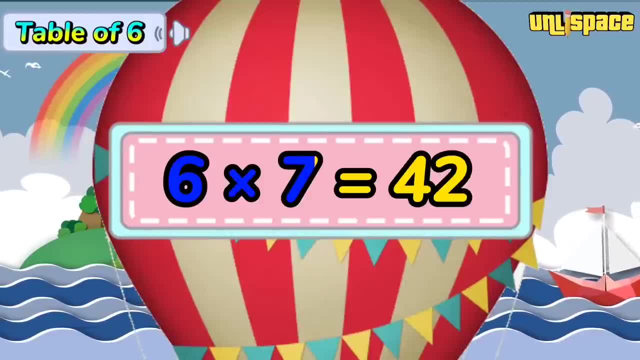 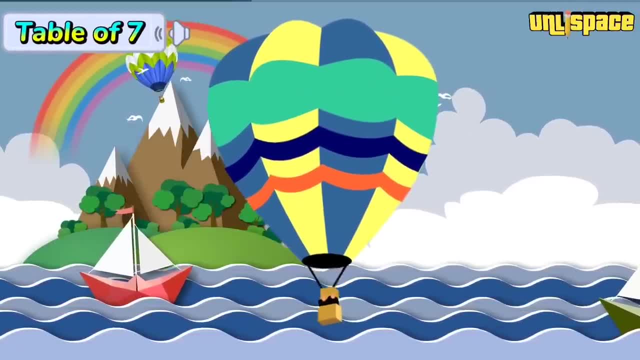 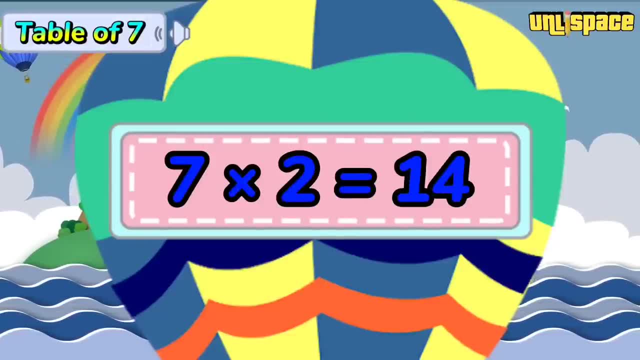 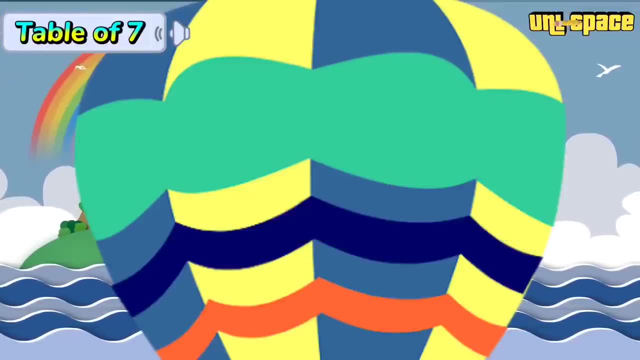 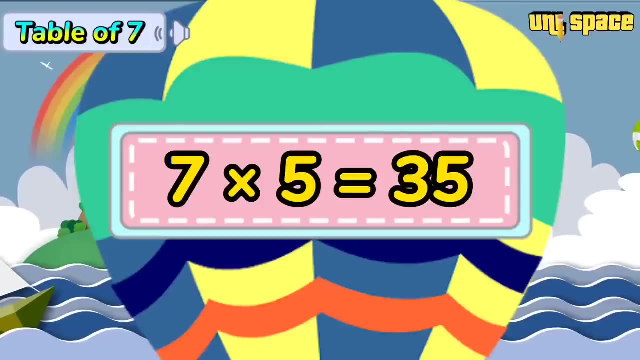 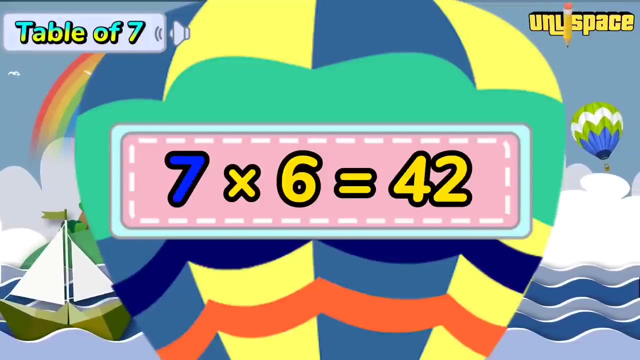 Six times ten equals forty-nine. Six times ten equals forty-nine. Six times ten equals forty-nine. Thanks for watching my video. If you like what you see, please, if you can give a thumbs up, subscribe To my channel. I have a lot of videos as well. Please do not Main yum. 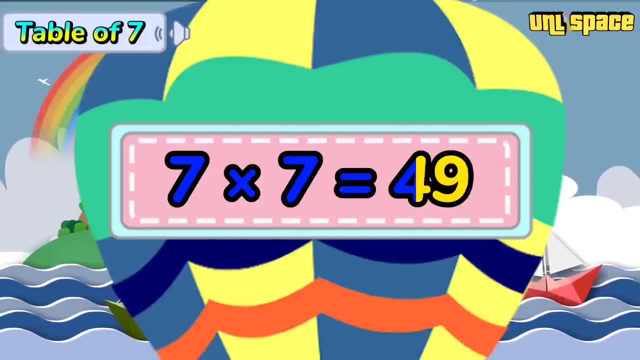 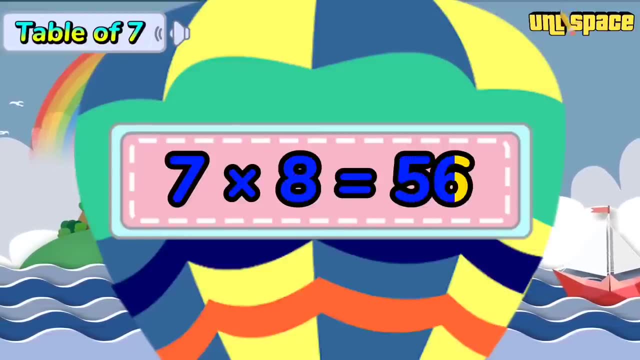 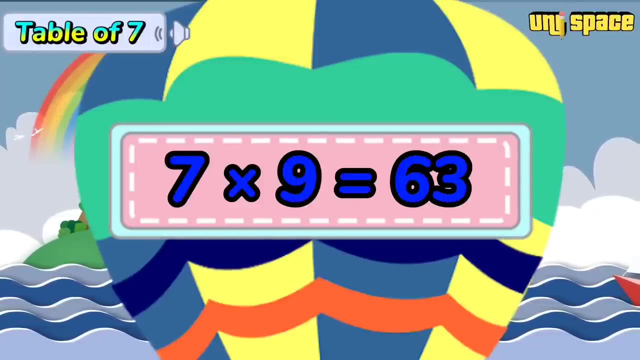 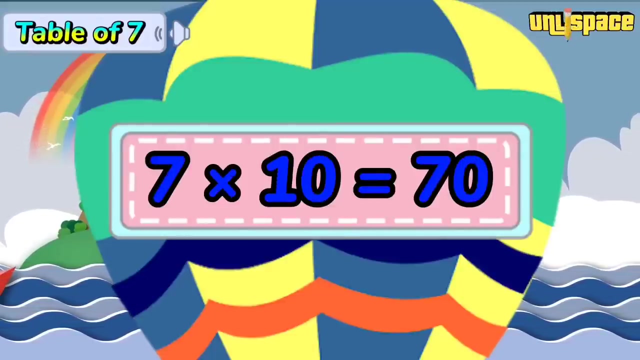 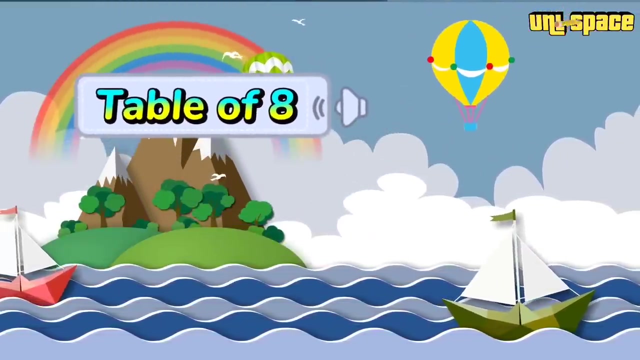 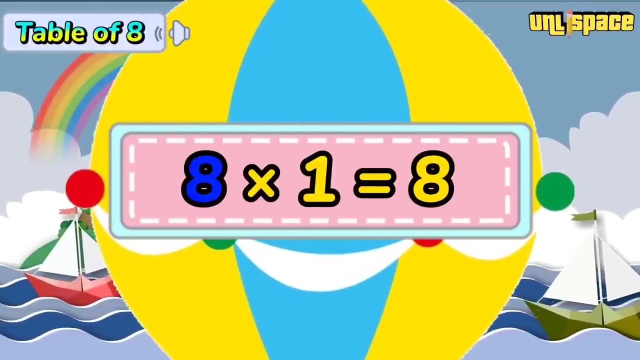 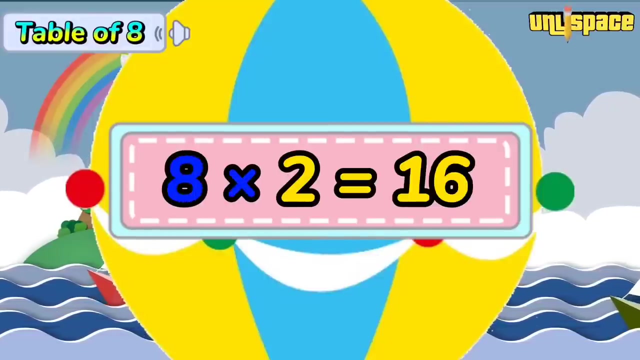 7 x 7 equals 49. 7 x 8 equals 56. 7 x 9 equals 63. 7 x 10 equals 70. 8 x 8 equals 20. 8 x 1 equals 8. 8 x 2 equals 16. 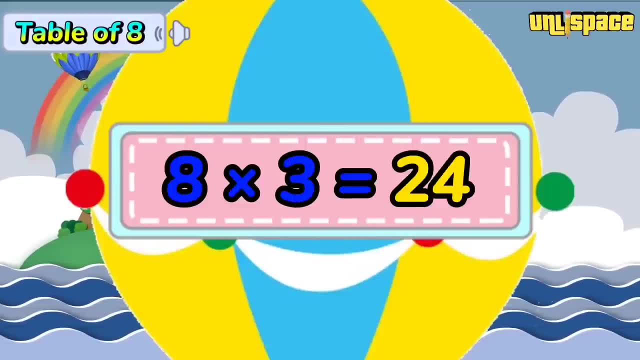 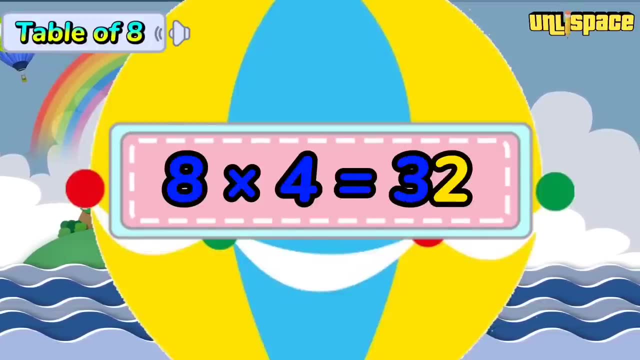 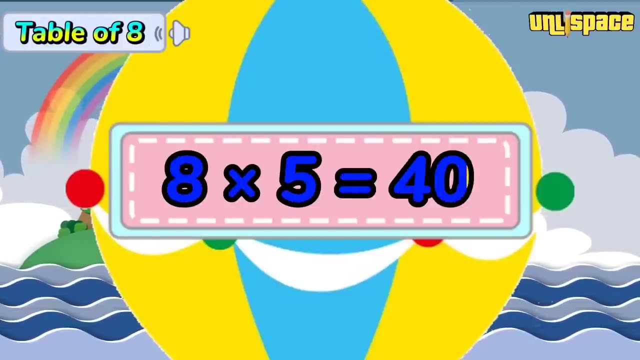 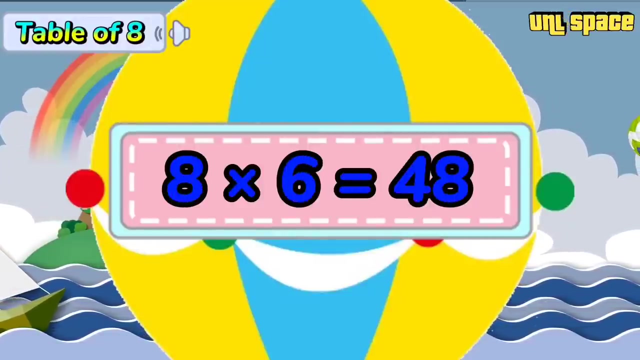 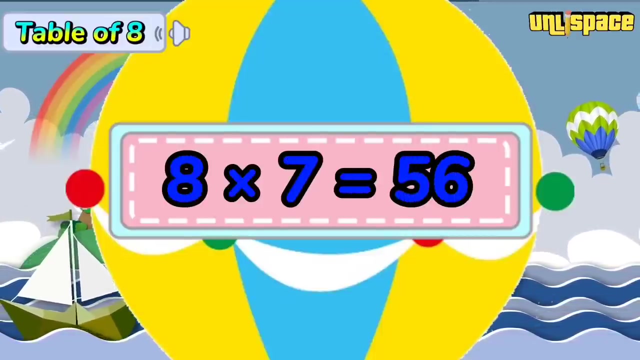 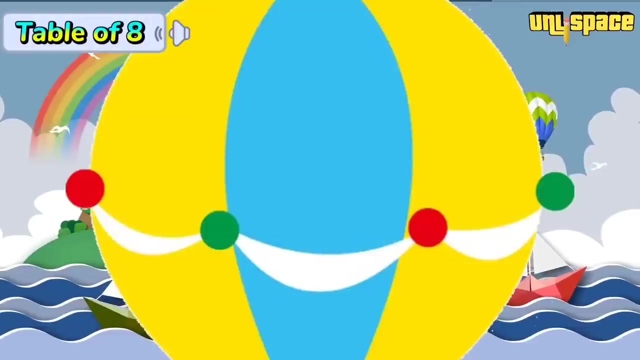 8 x 3 equals 24. 8 x 4 equals 32. 8 x 5 equals 40. 8 x 6 equals 48. 8 x 7 equals 56. 8 x 8 equals 64. 8 x 9 equals 72. 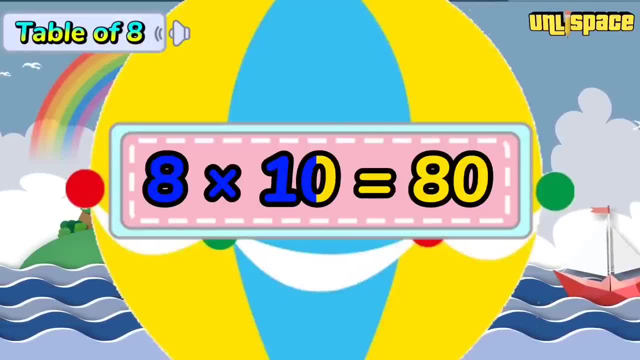 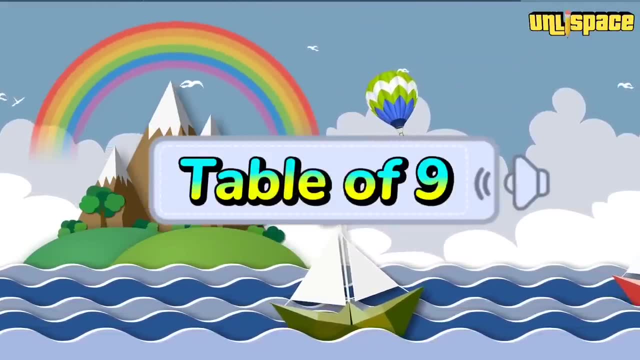 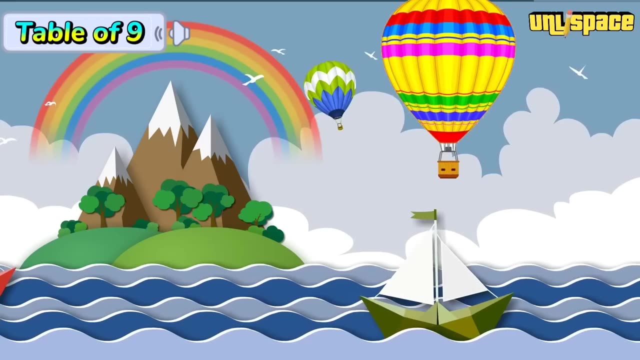 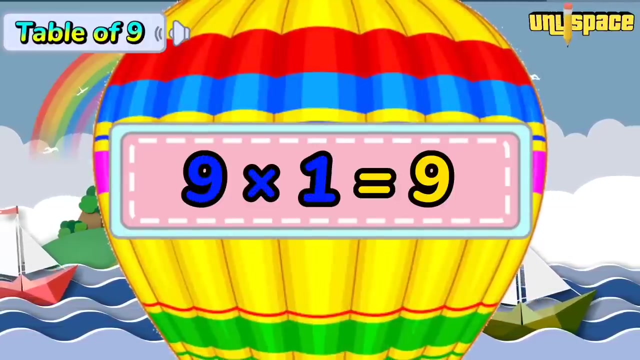 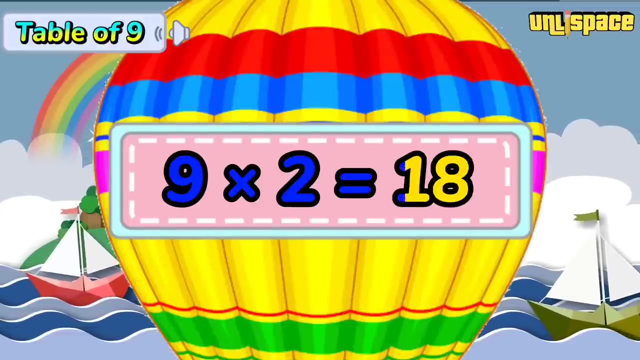 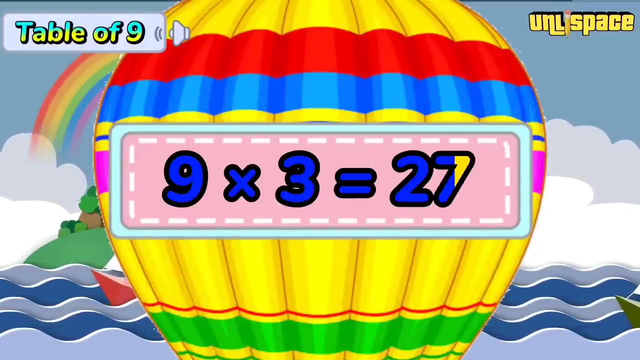 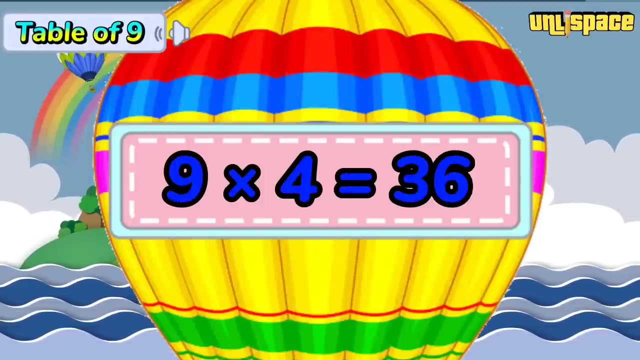 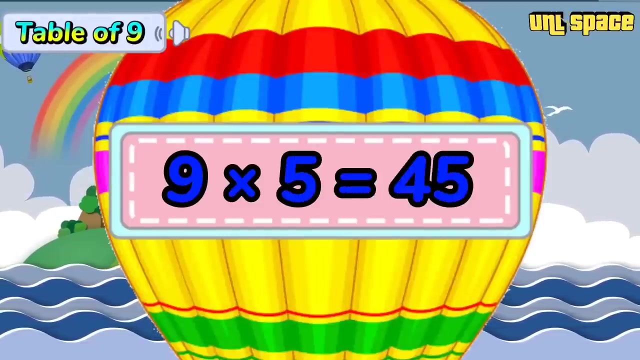 8 x 10 equals 80. Table of Nine: 9 x 1 equals 9. 9 x 2 equals 18. 9 x 3 equals 27. 9 x 4 equals 36. 9 x 5 equals 45. 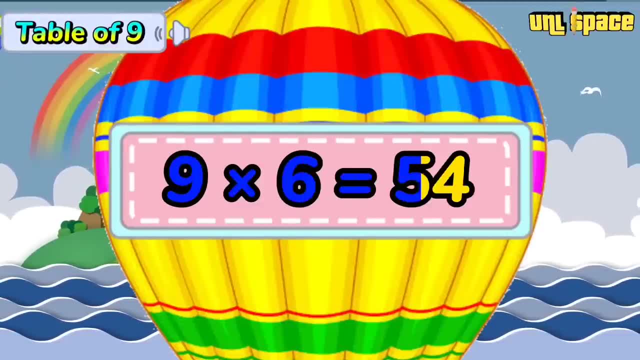 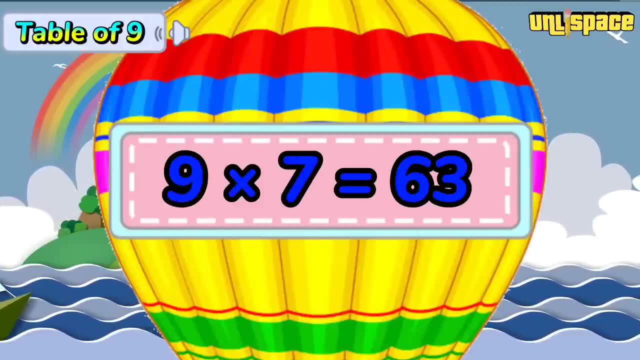 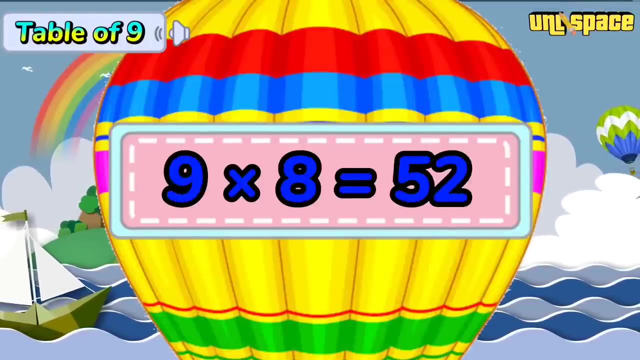 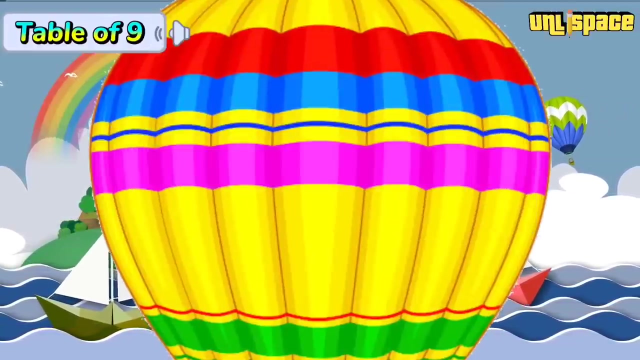 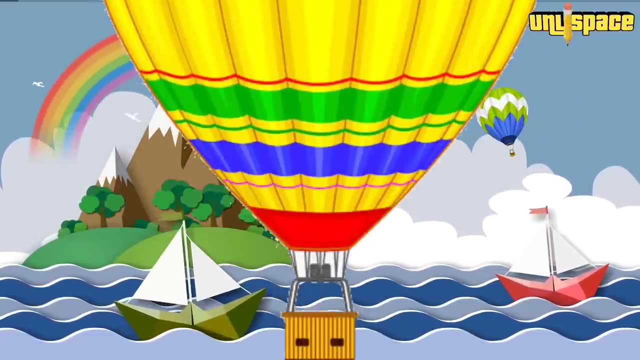 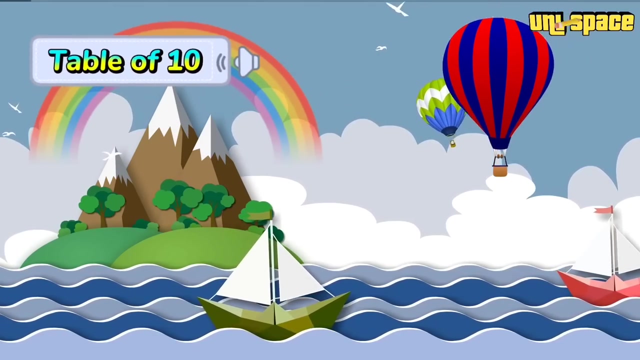 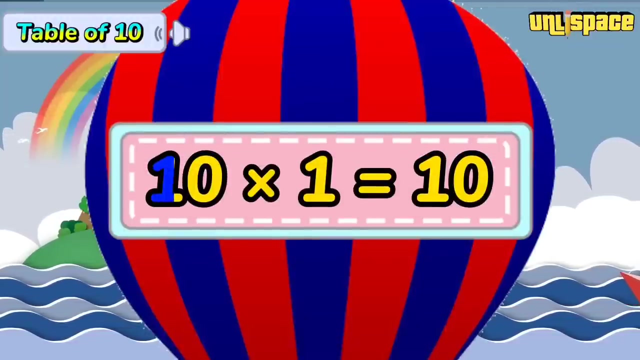 9 x 6 equals 54. 9 x 7 equals 63. 9 x 8 equals 52. 9 x 9 equals 61. 9 x 10 equals 90. Table of Ten: 10 x 1 equals 10. 10 x 2 equals 32. 10 x 3 equals 32. 10 x 4 equals 32. 10 x 3 equals 32. 10 x 4 equals 30. 10 x 4 equals 40. 10 x 5 equals 50. 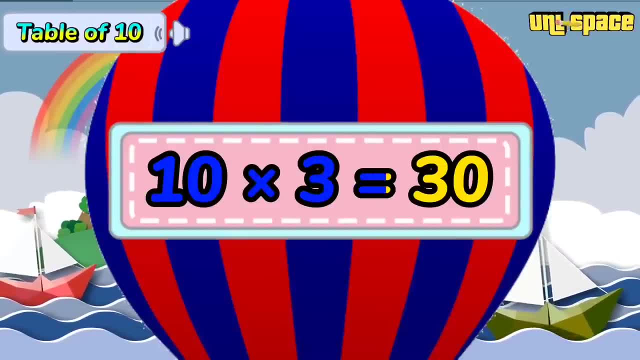 10 x 5 equals 50. 10 x 6 equals 60. 10 x 6 equals 60. 10 x 7 equals 60. 10 x 8 equals 60. 10 x 9 equals 60. 10 x 9 equals 60. 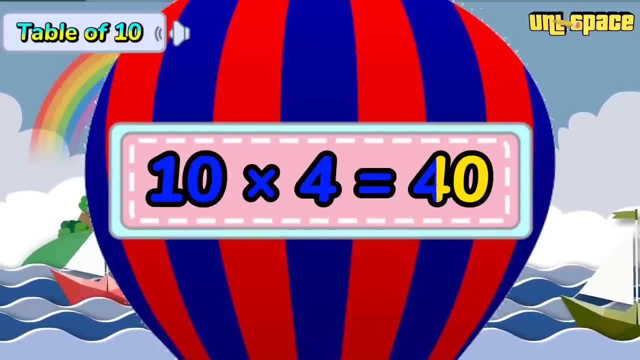 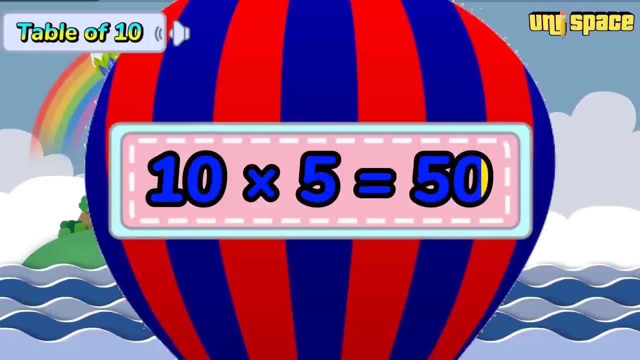 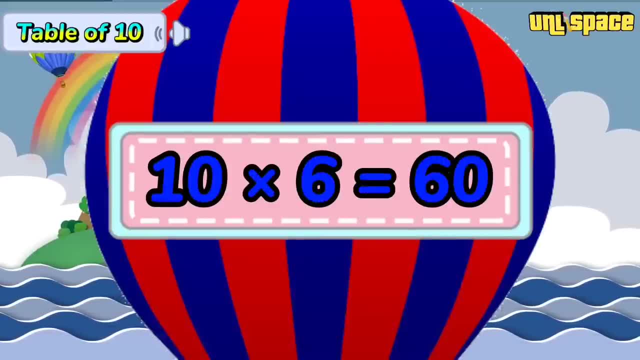 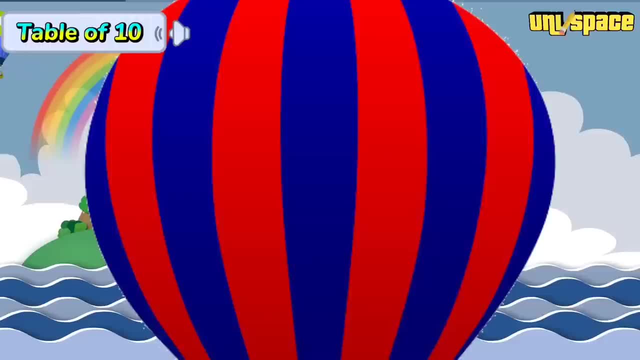 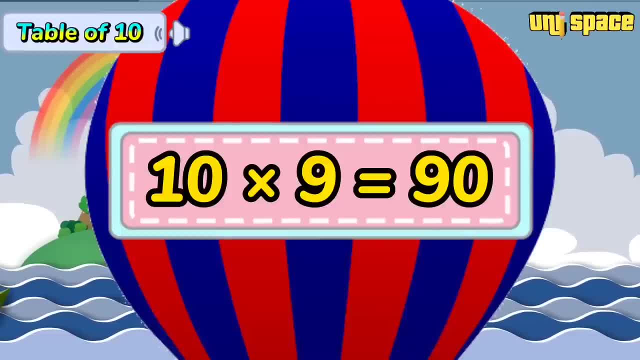 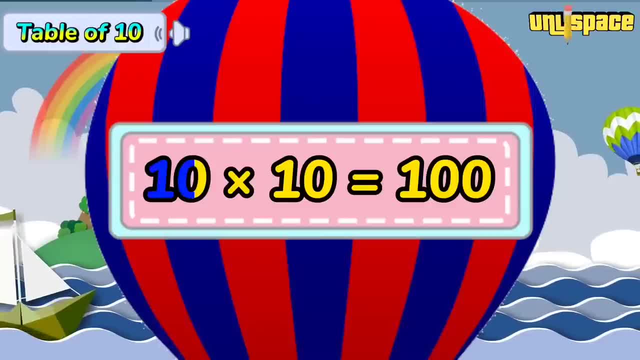 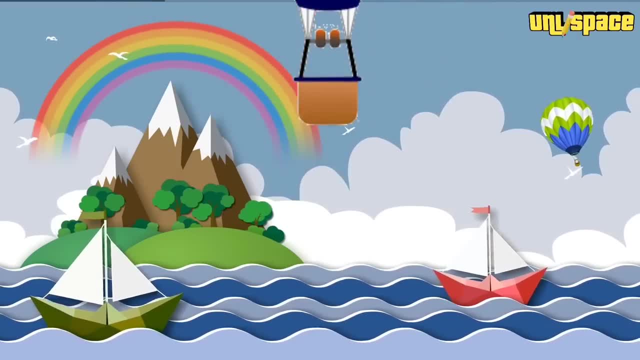 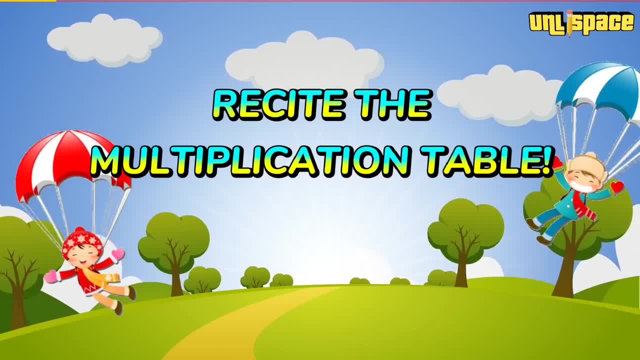 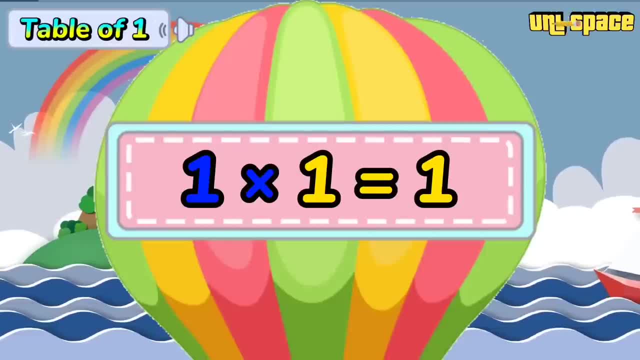 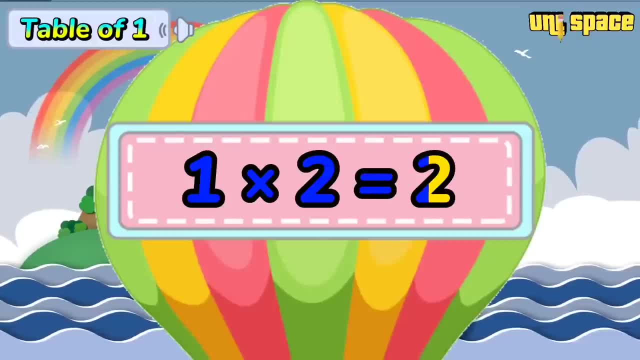 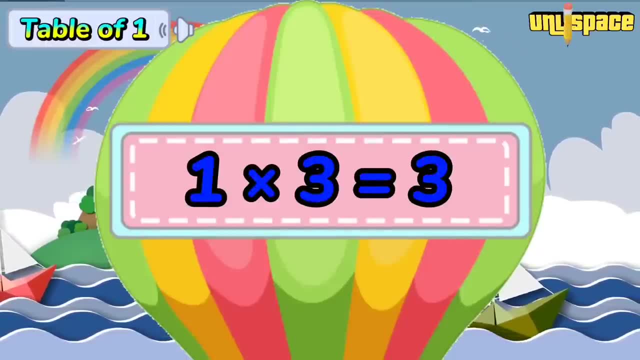 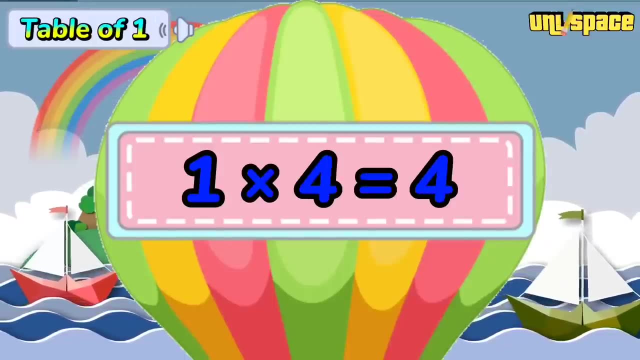 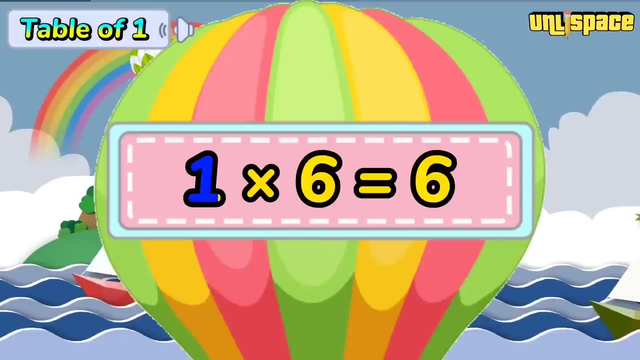 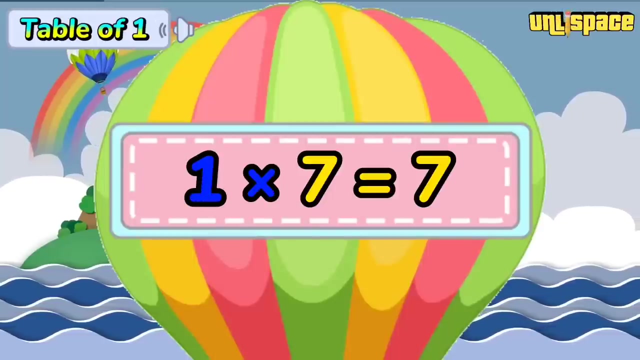 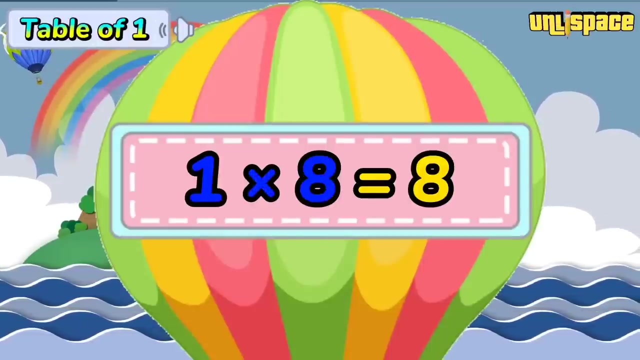 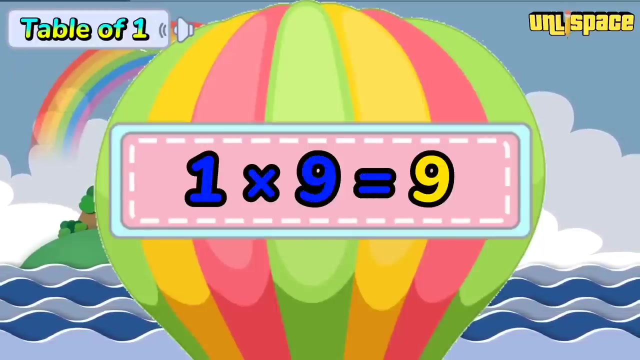 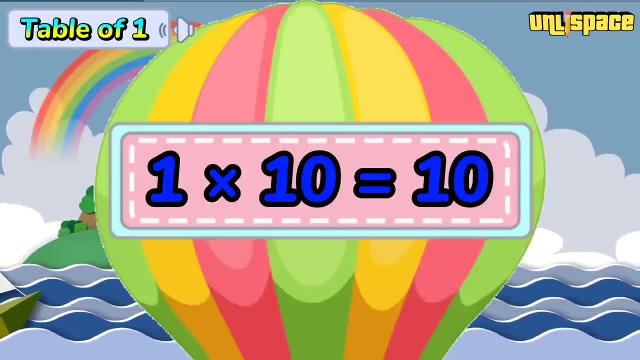 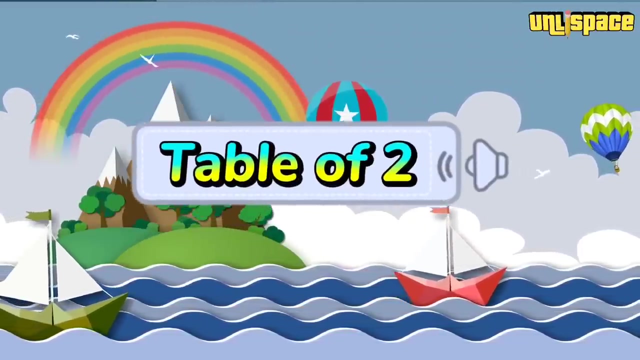 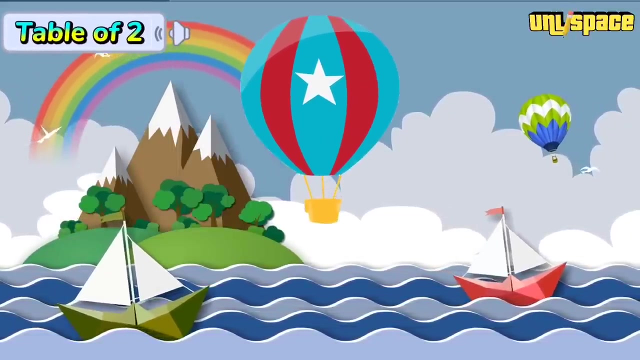 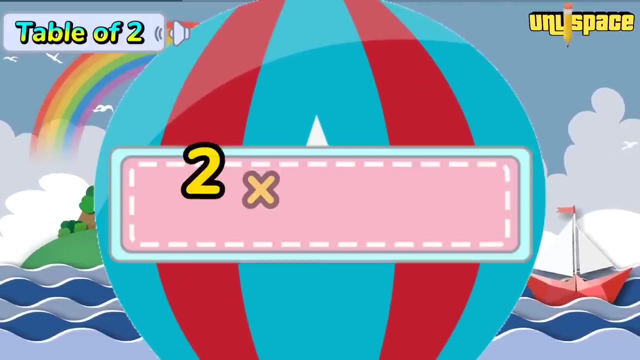 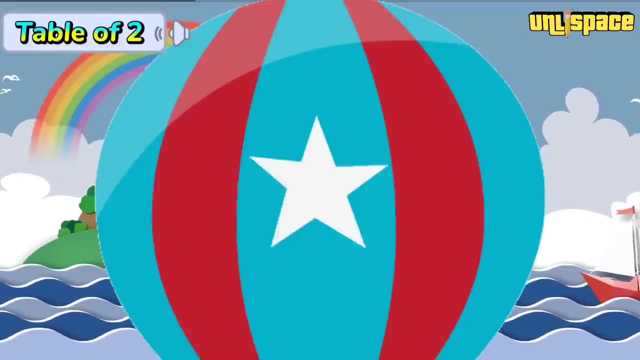 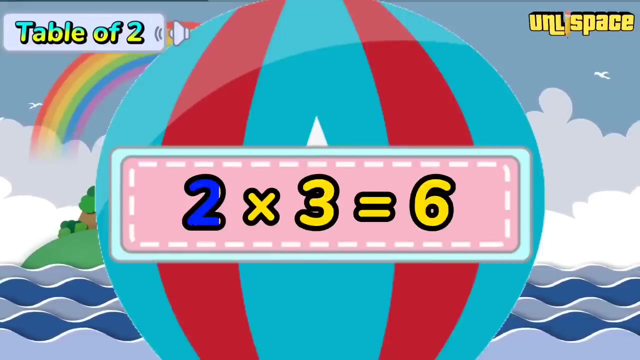 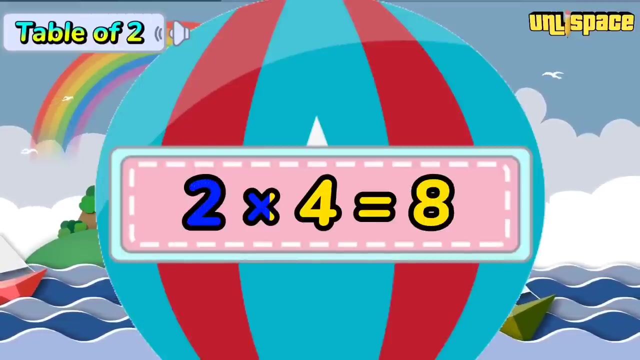 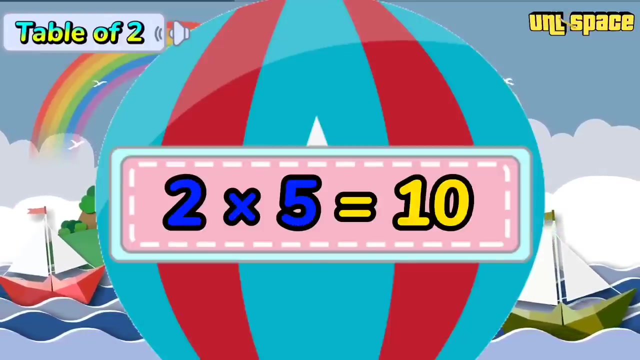 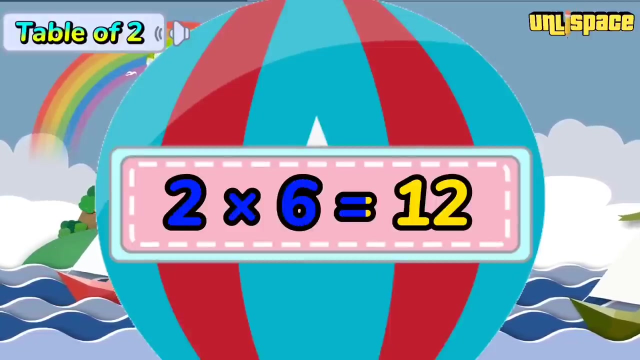 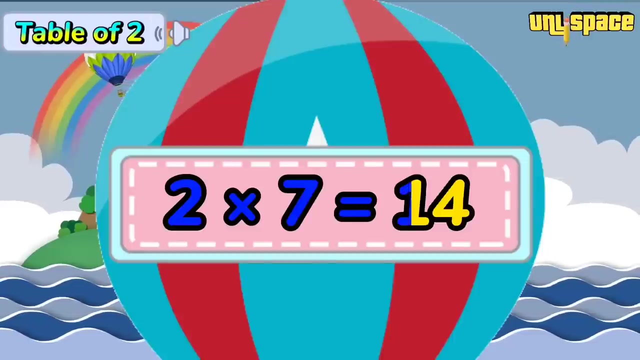 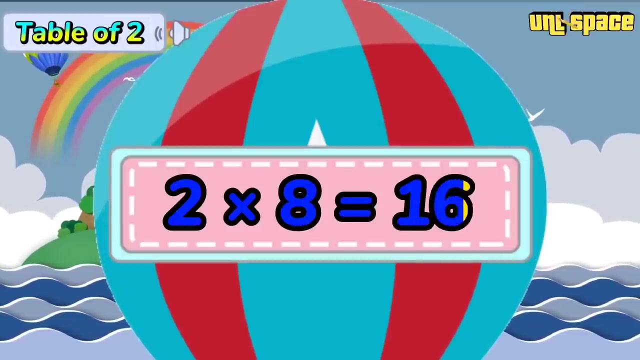 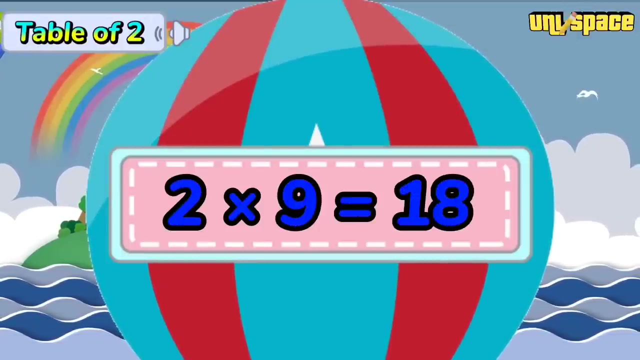 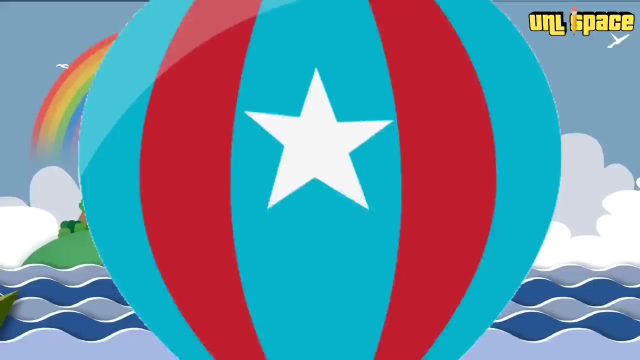 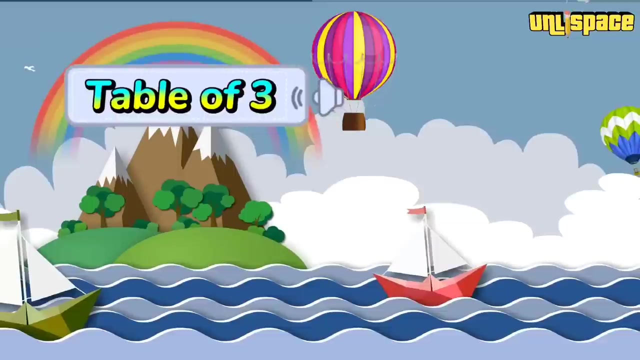 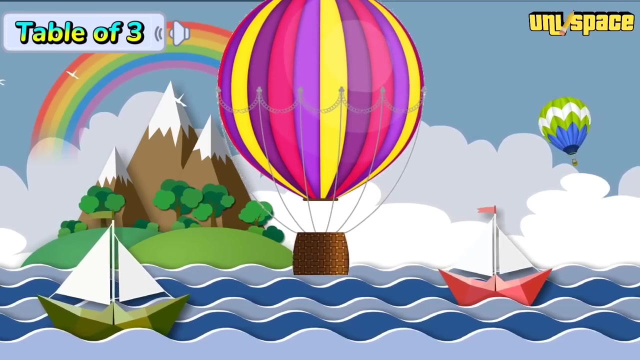 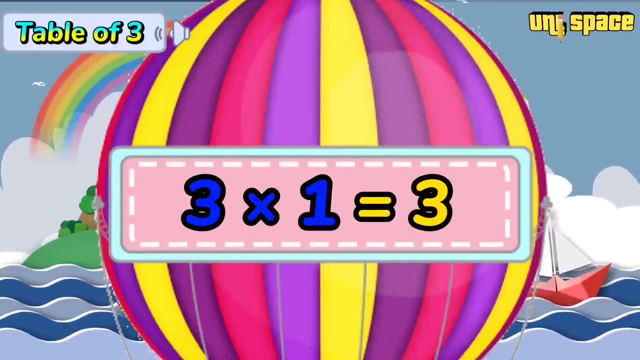 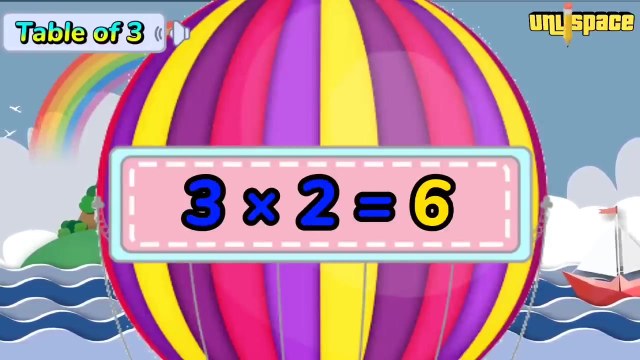 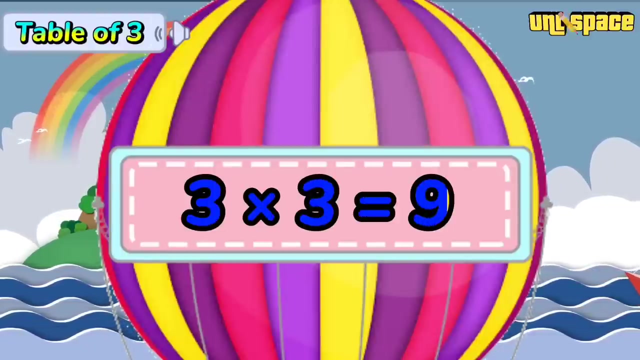 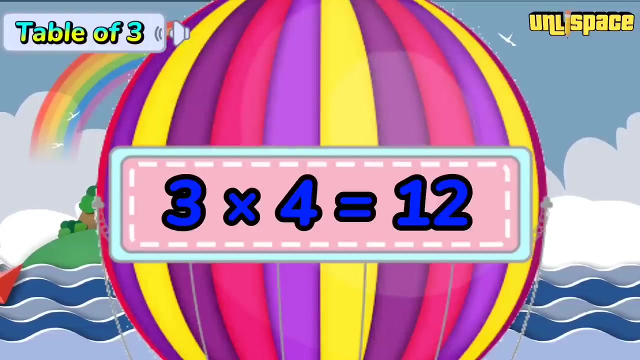 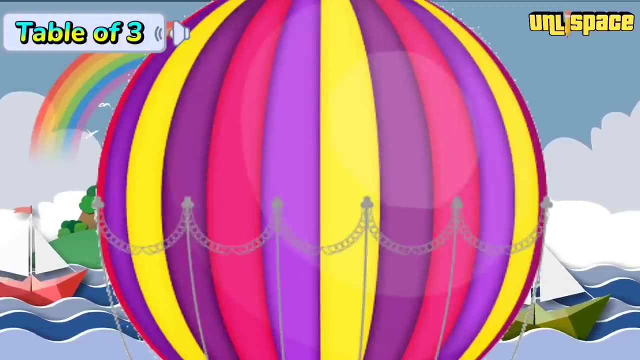 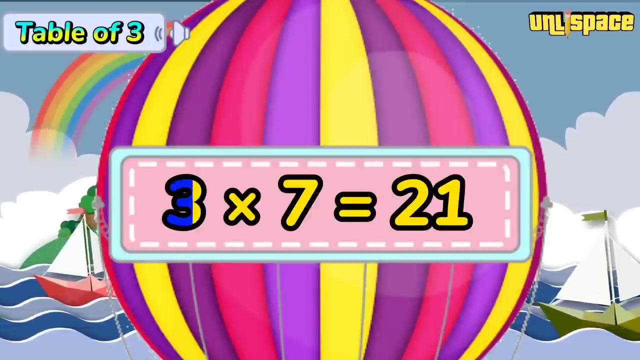 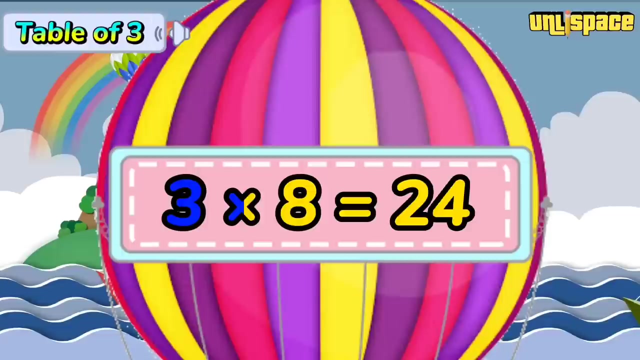 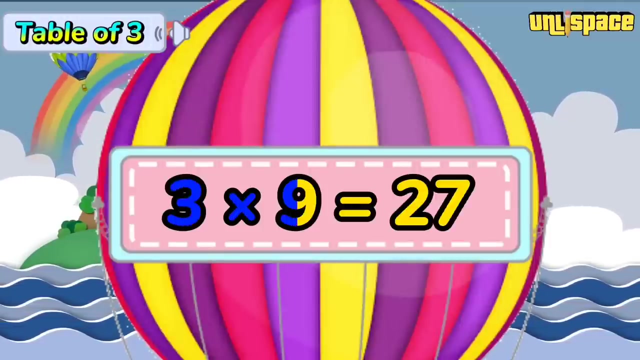 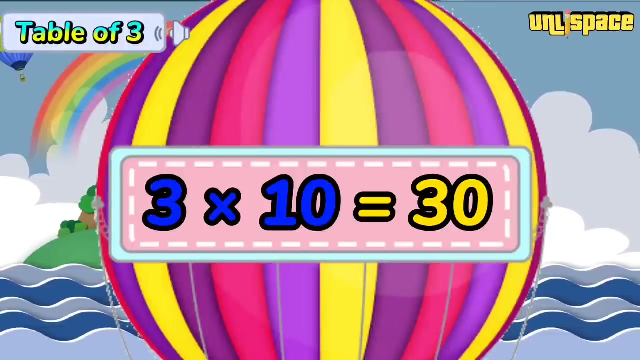 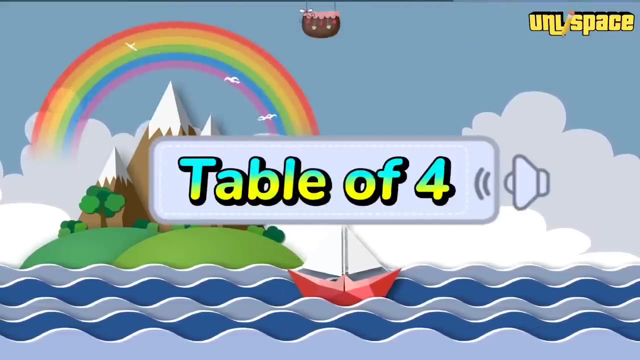 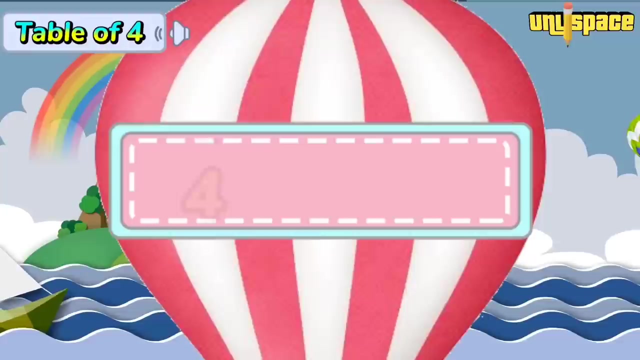 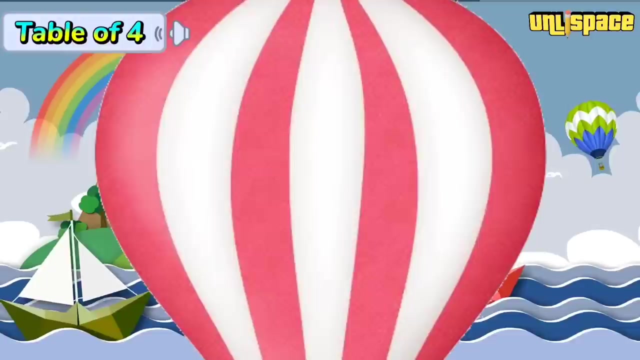 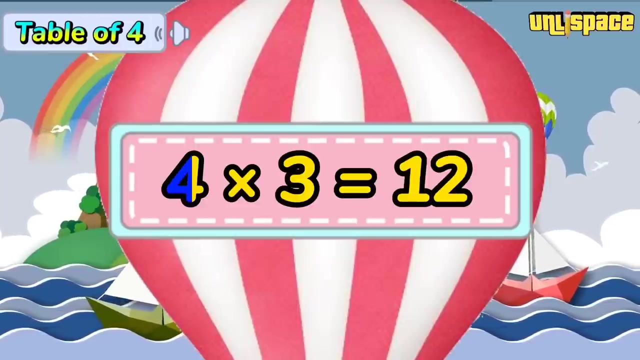 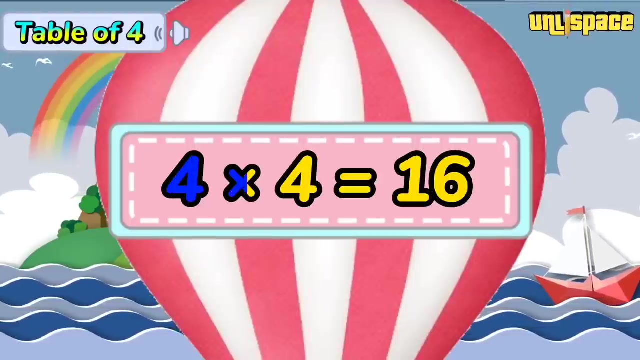 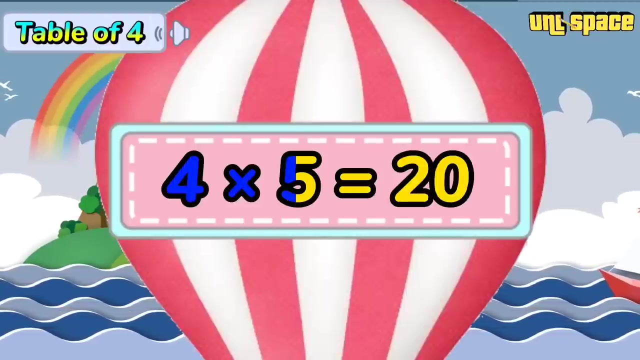 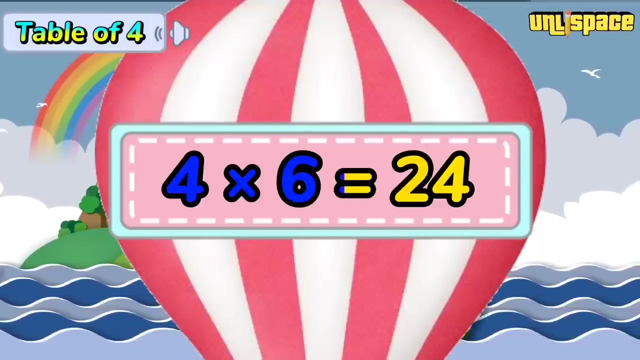 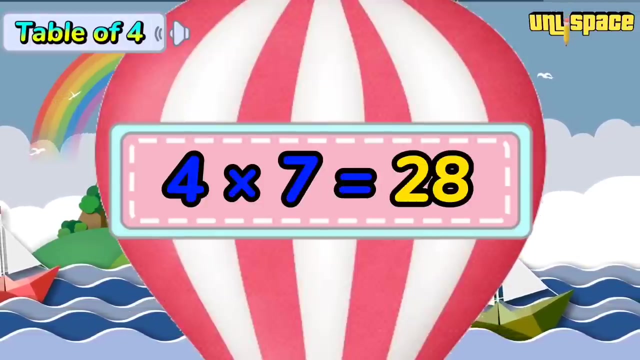 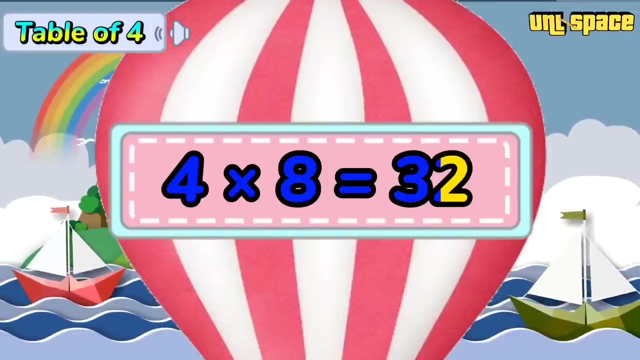 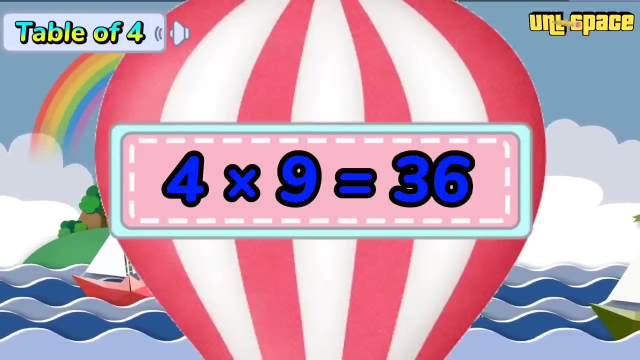 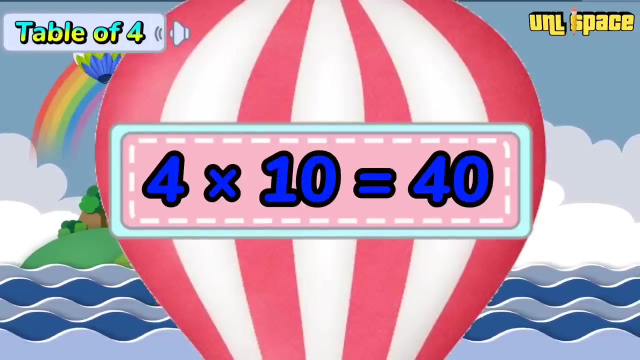 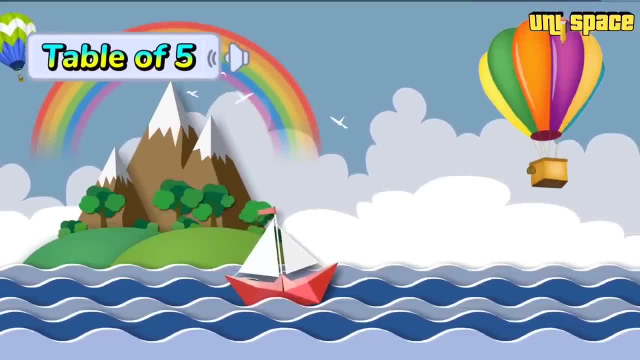 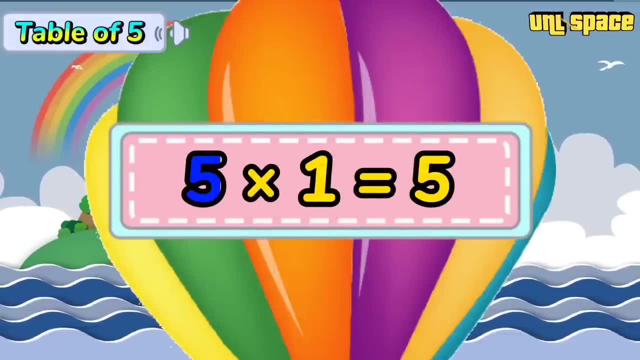 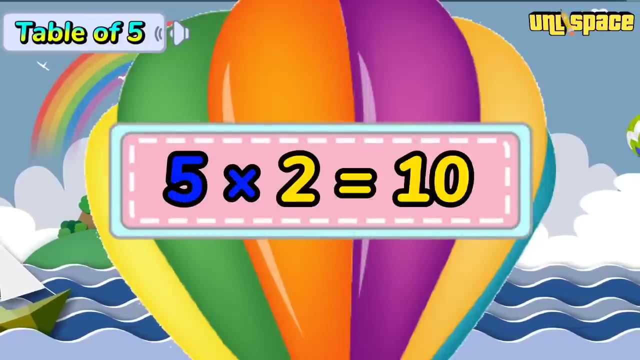 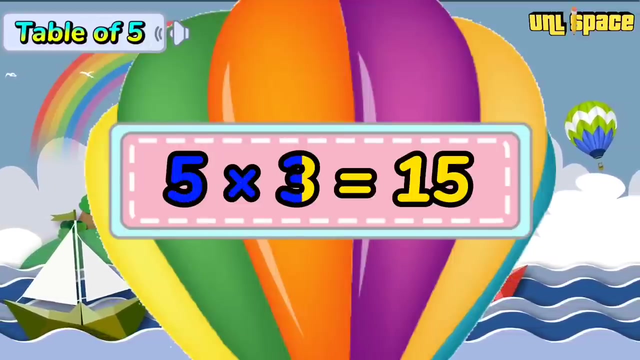 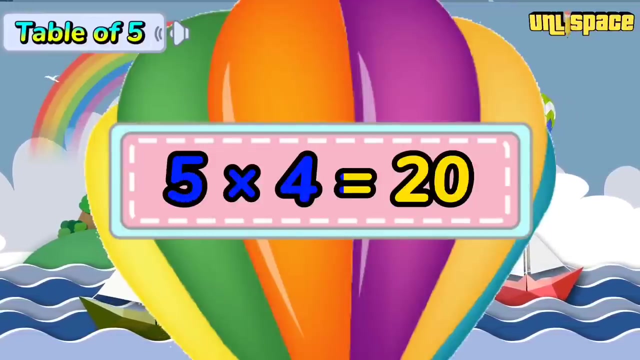 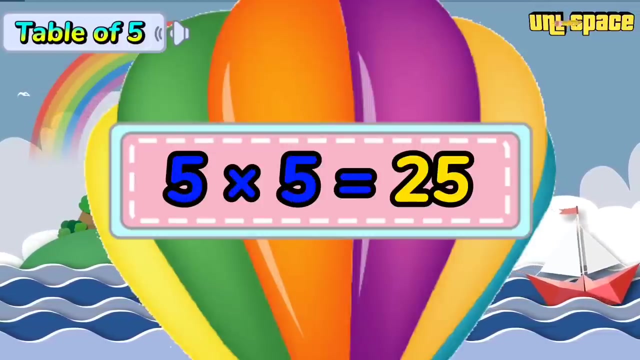 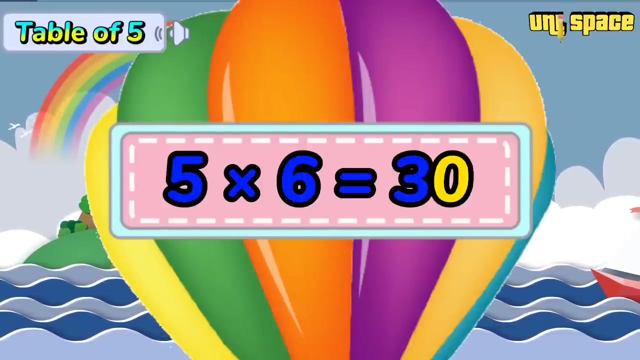 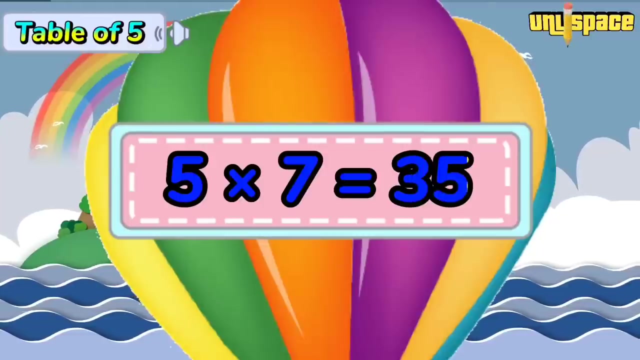 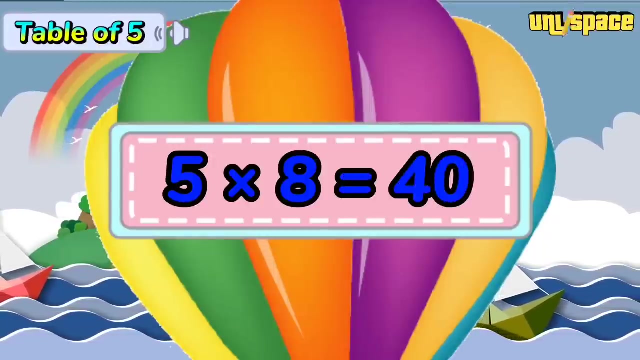 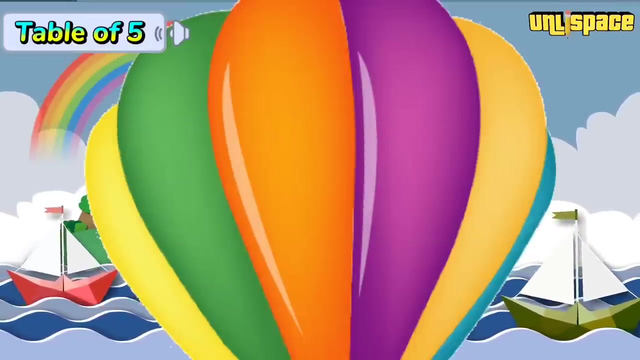 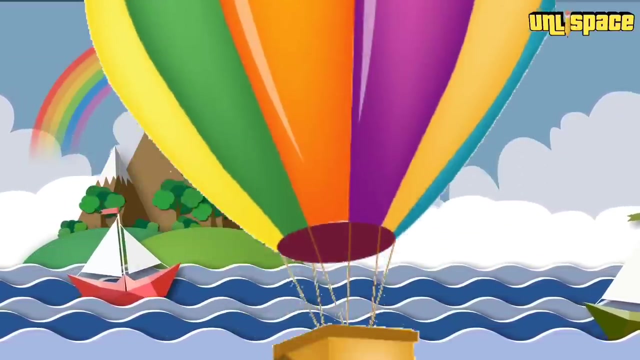 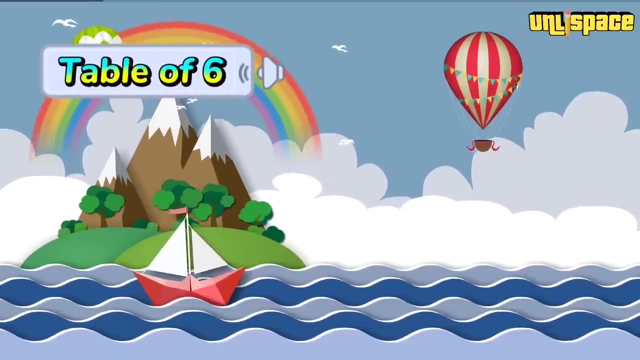 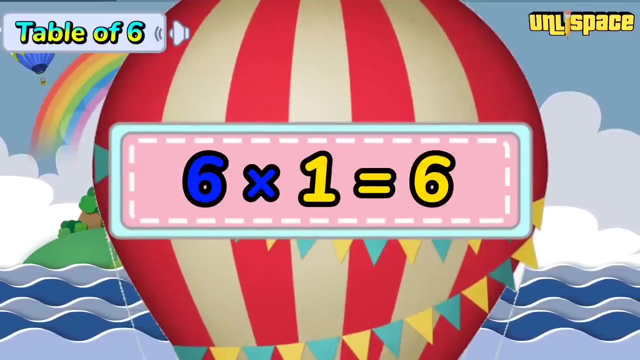 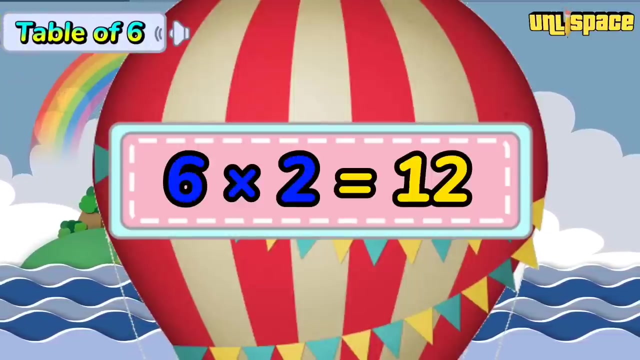 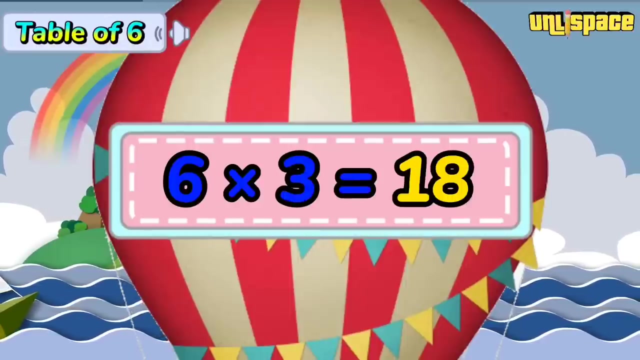 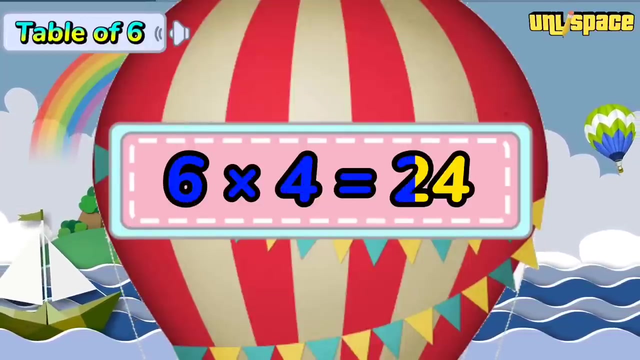 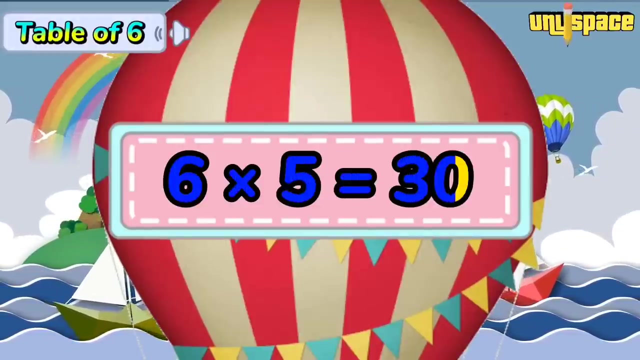 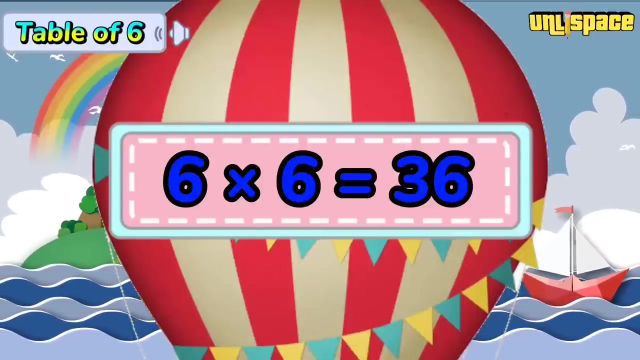 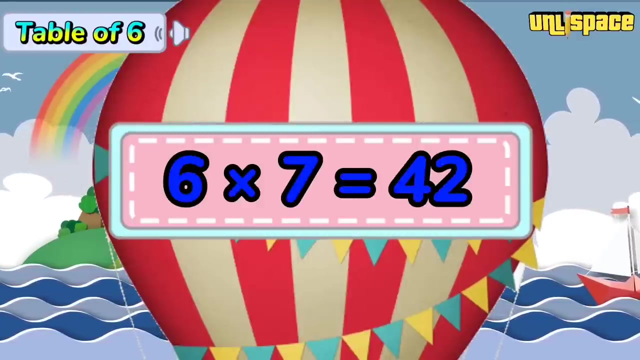 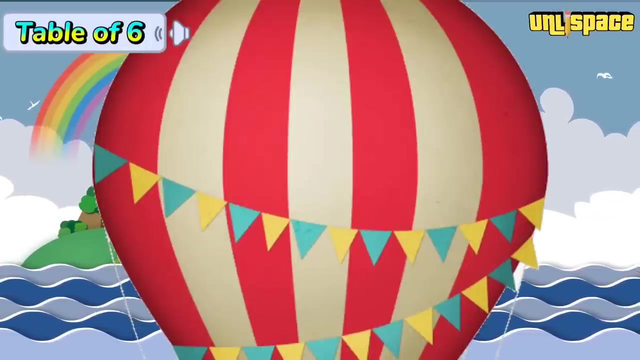 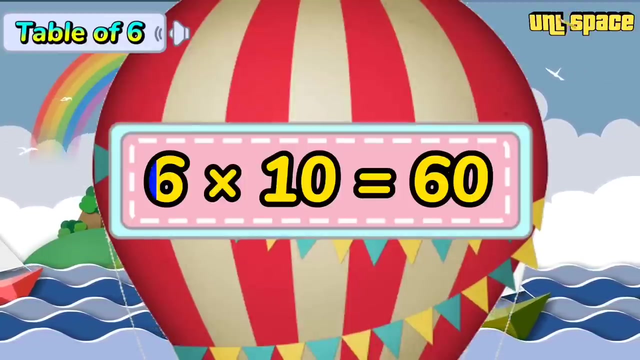 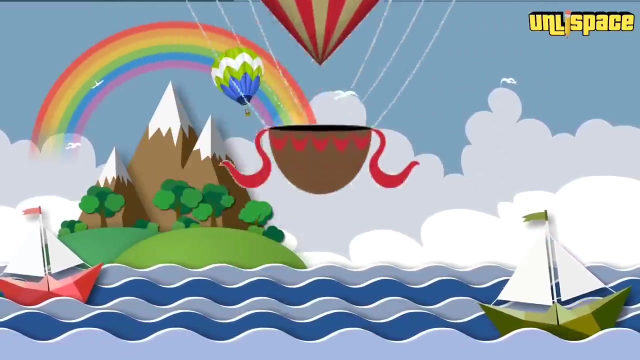 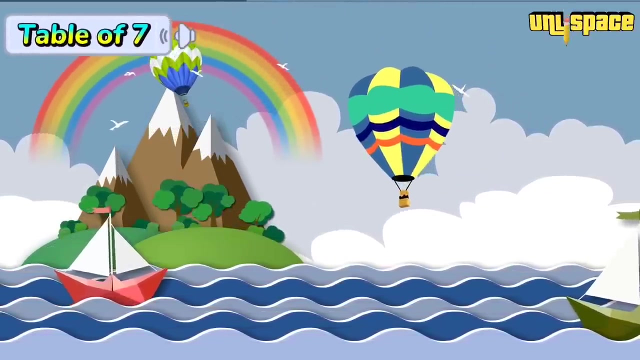 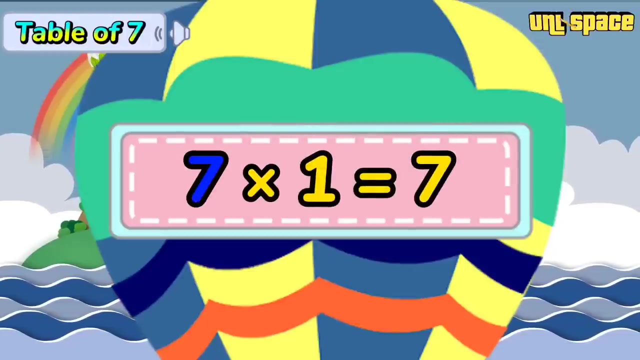 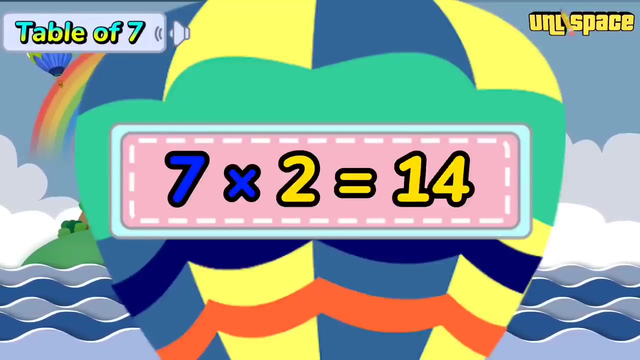 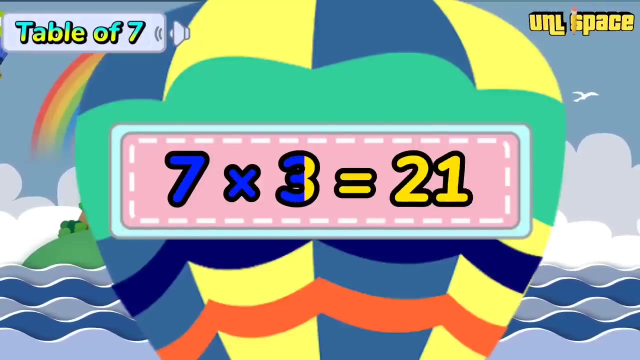 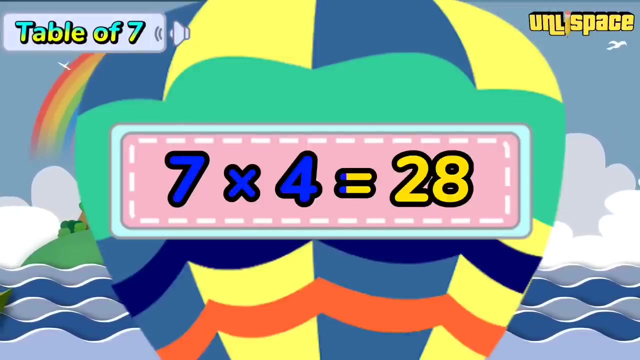 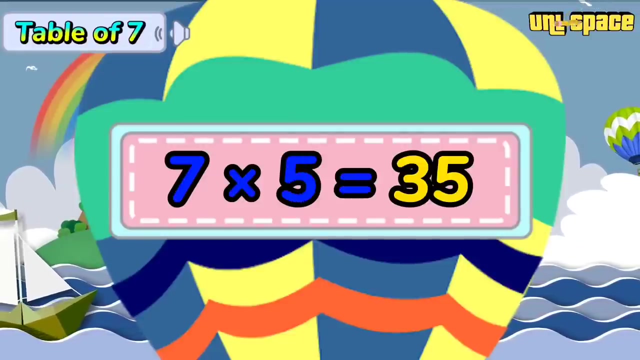 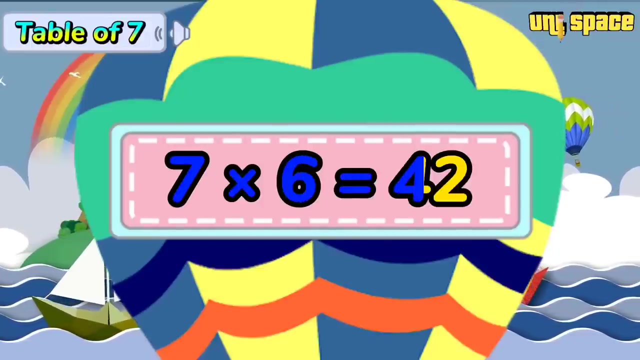 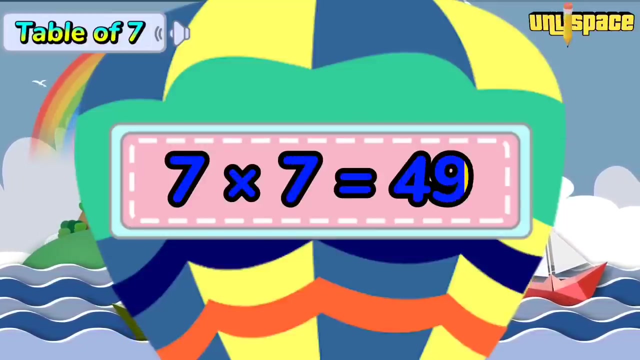 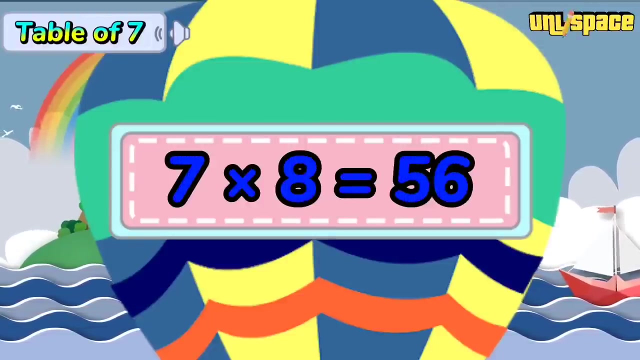 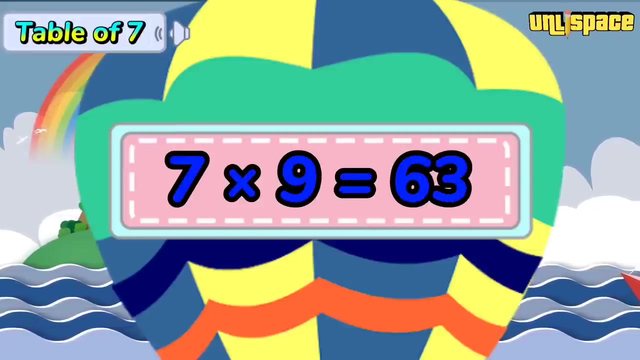 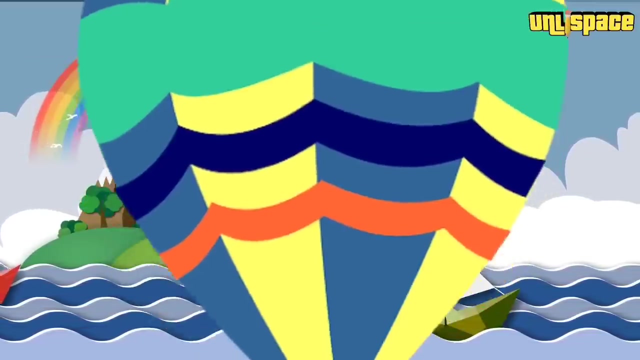 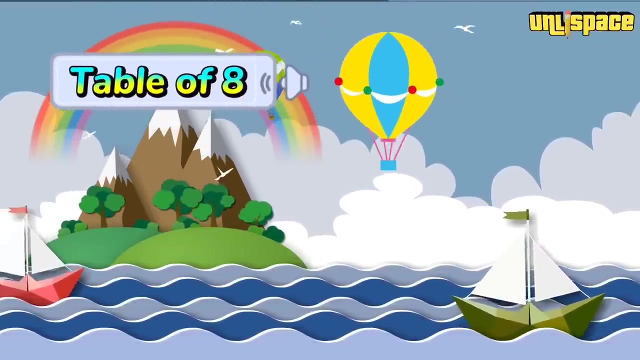 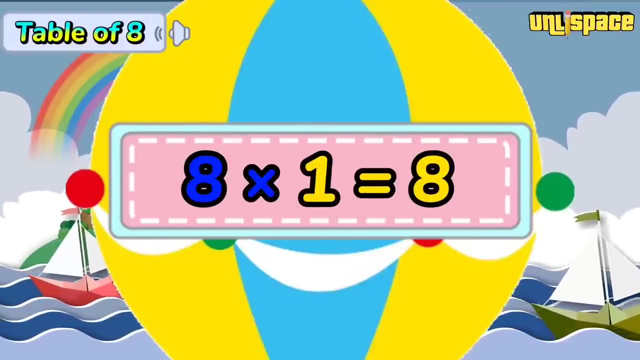 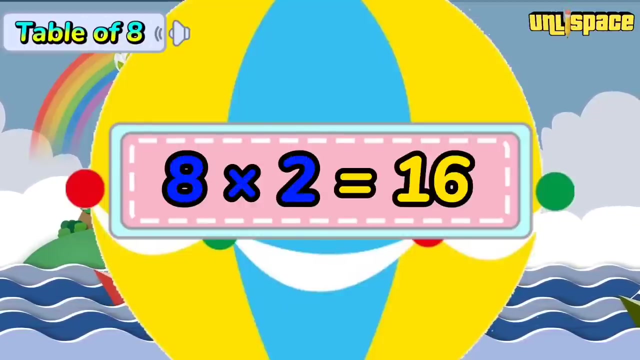 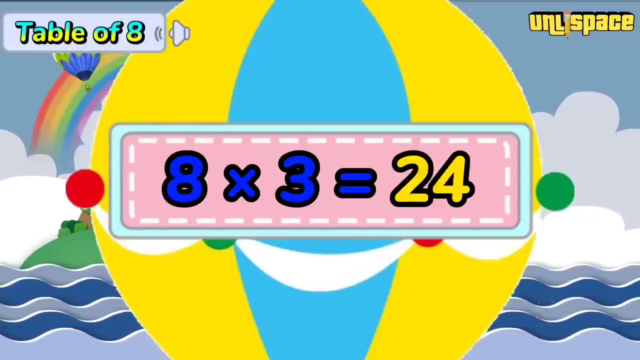 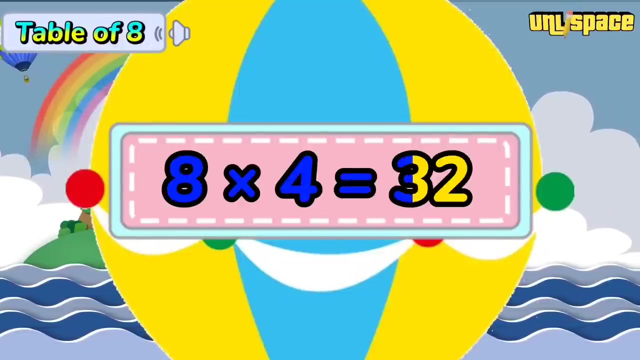 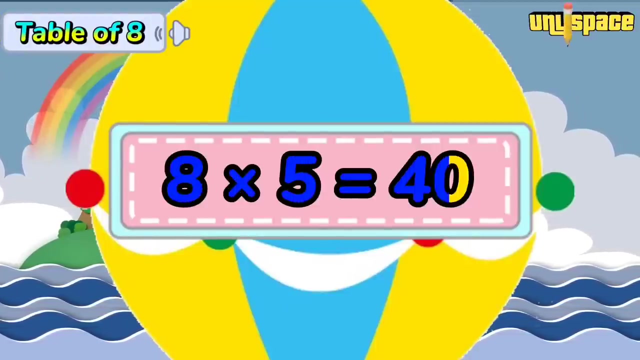 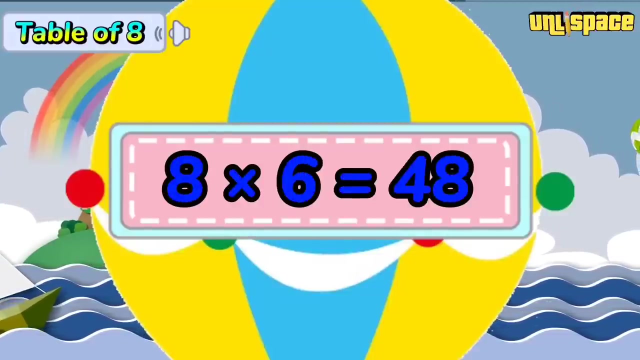 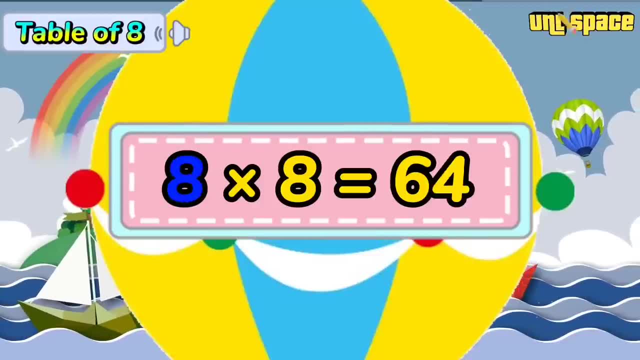 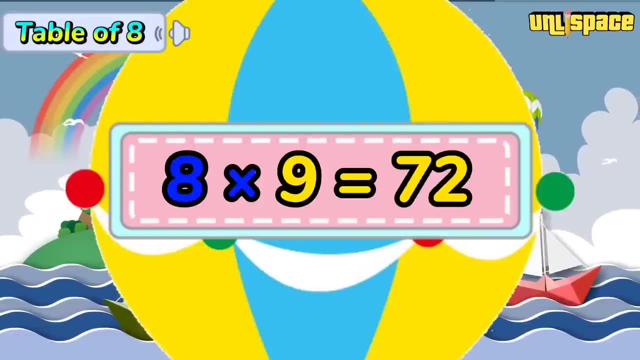 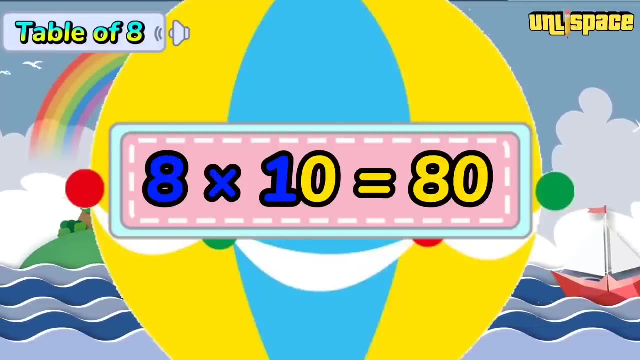 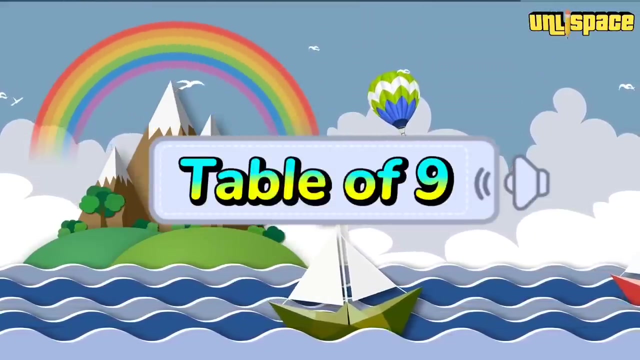 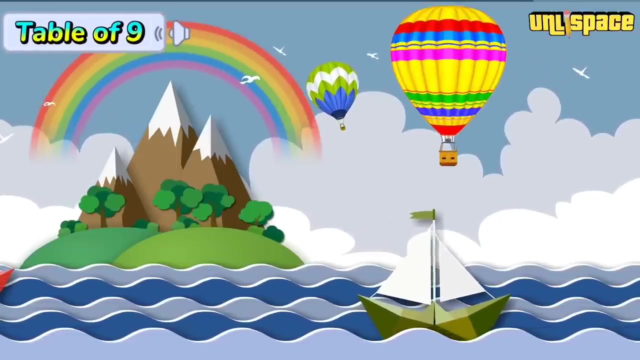 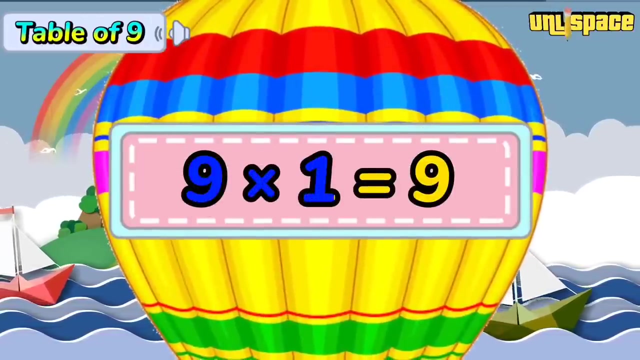 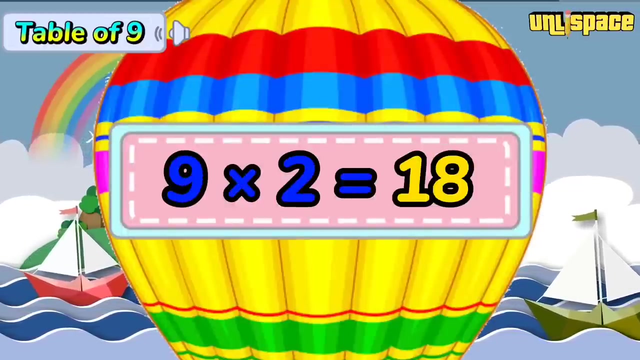 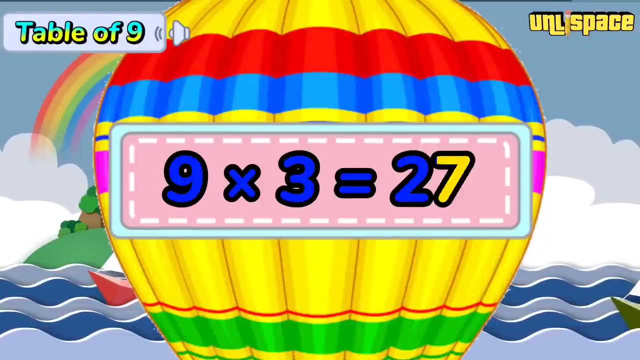 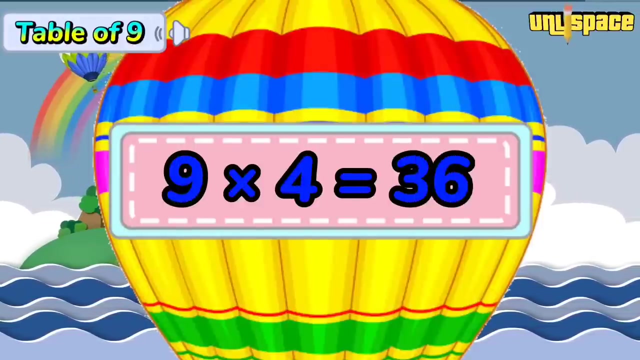 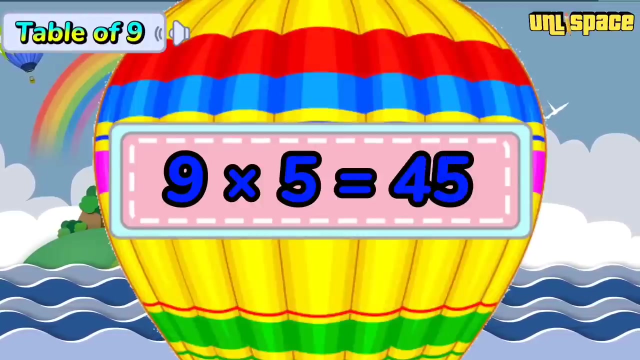 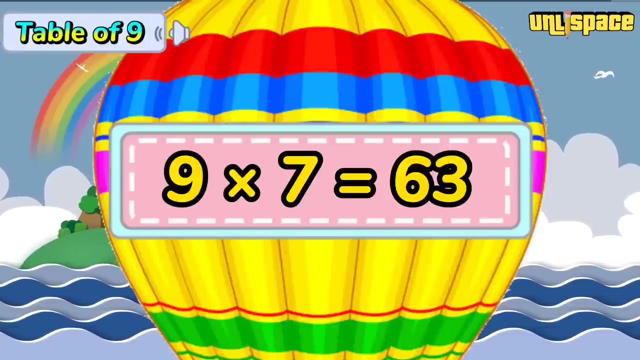 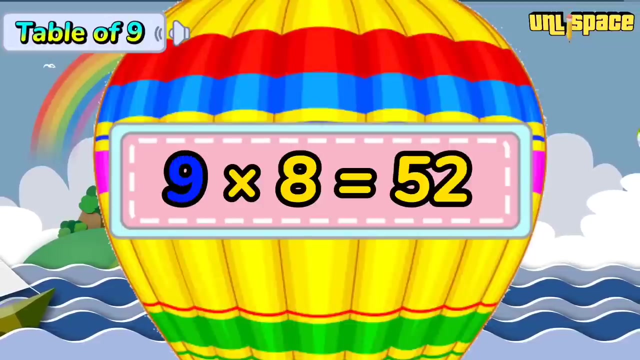 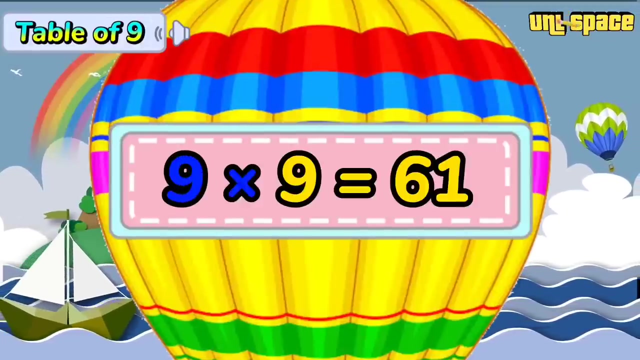 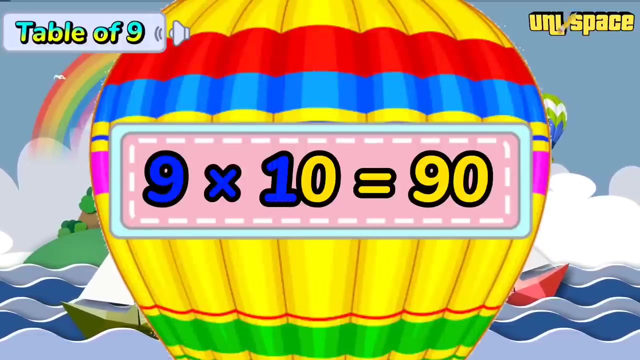 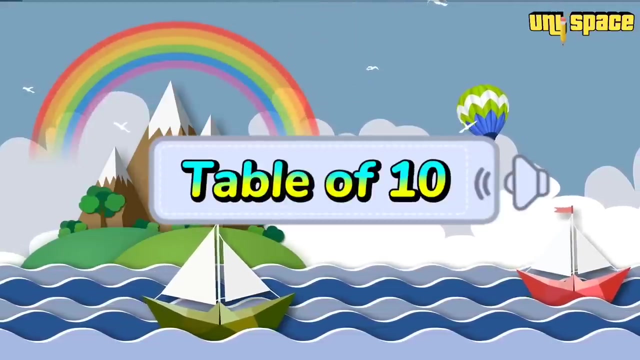 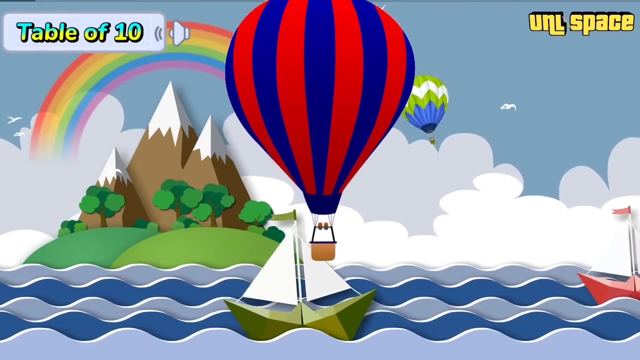 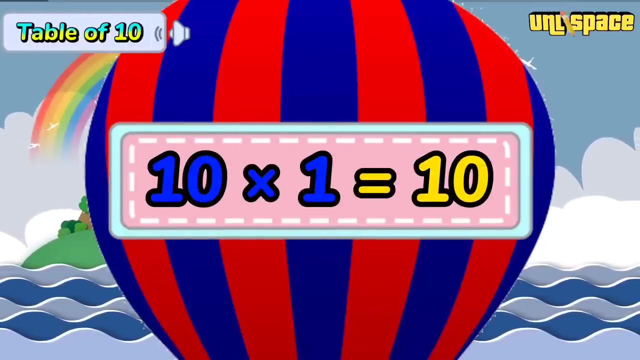 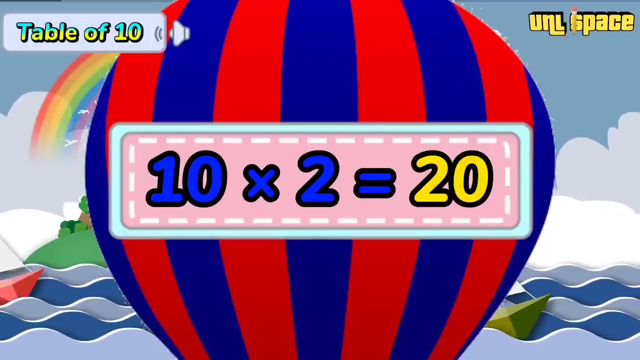 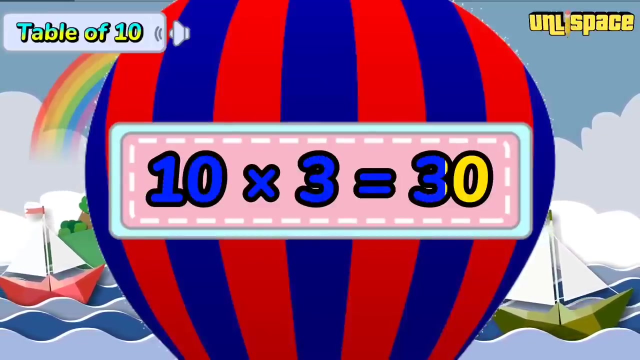 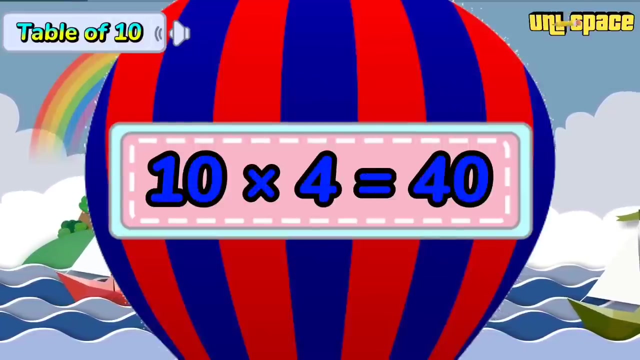 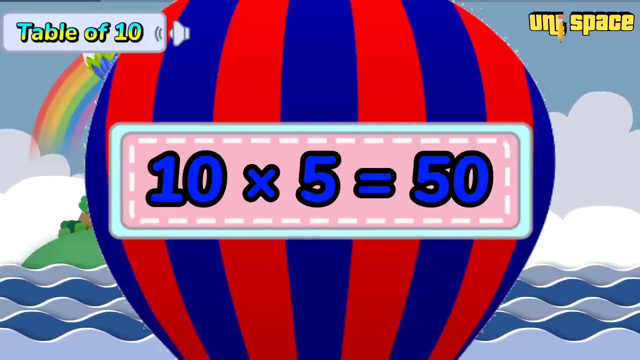 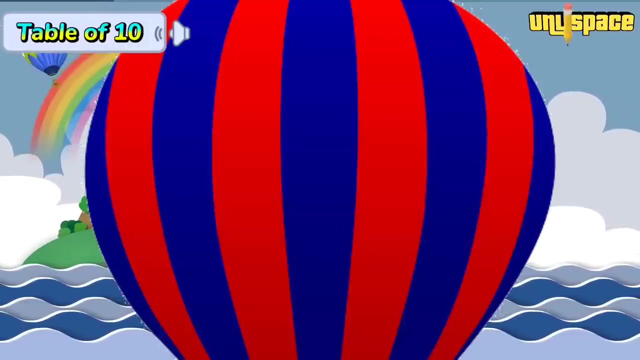 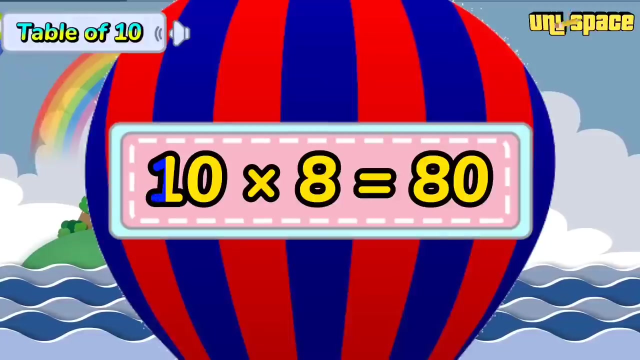 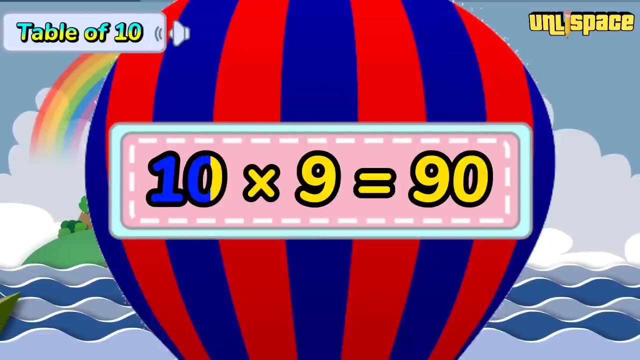 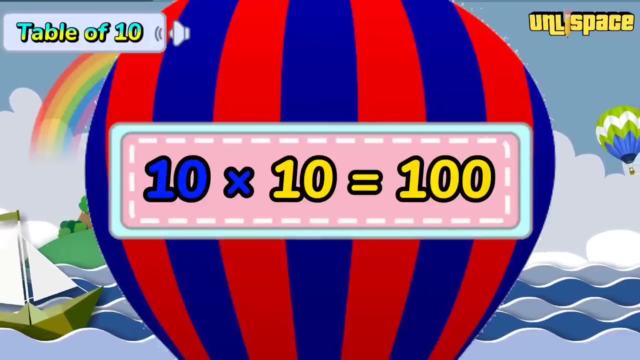 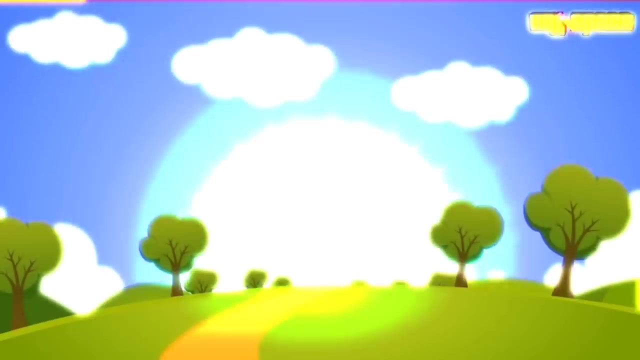 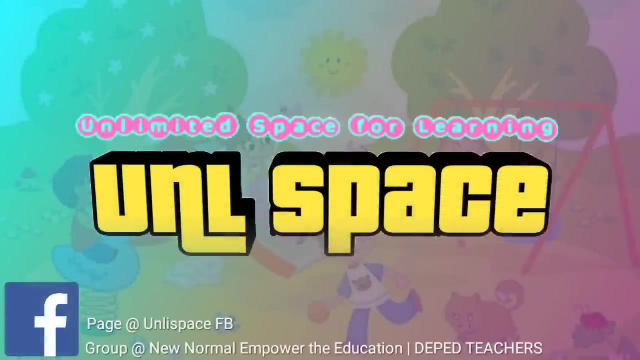